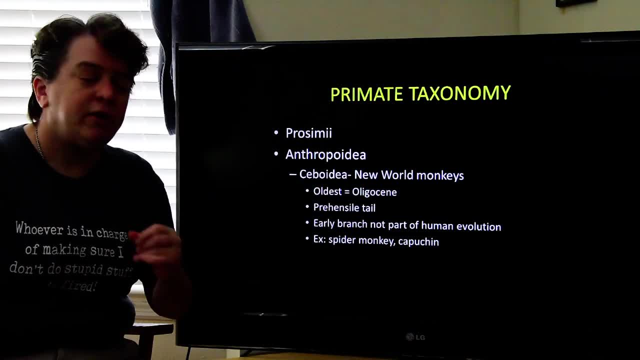 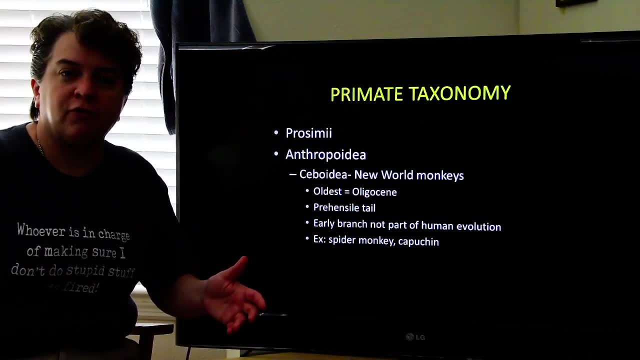 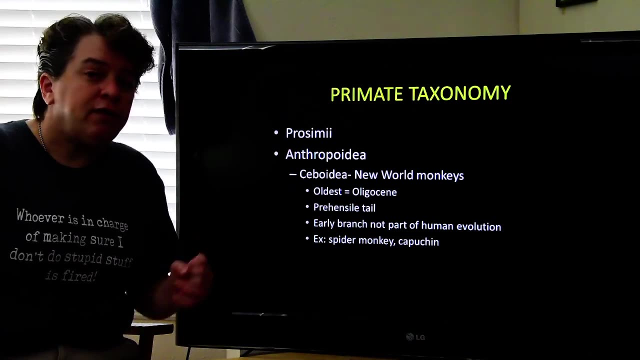 In anthropoidea we have seboidea. These are new world monkeys. So if you go down to the Amazon rainforest or parts of Central America and you see little monkeys running around in the trees, that is our new world monkeys. The oldest that we know of is in the Oligocene. These monkeys have a prehensile tail, so they 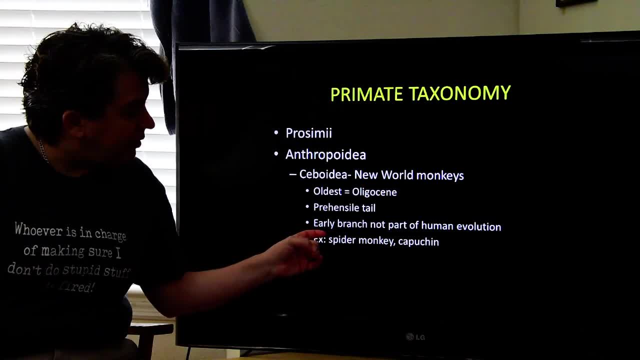 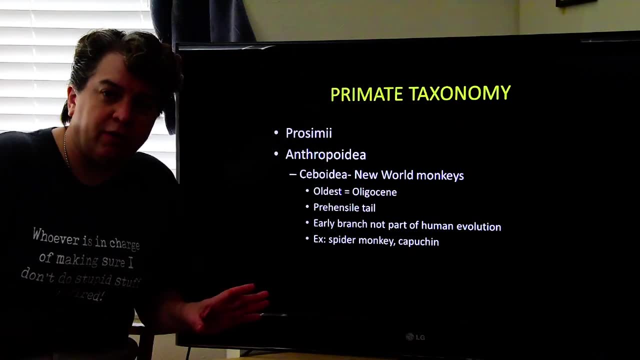 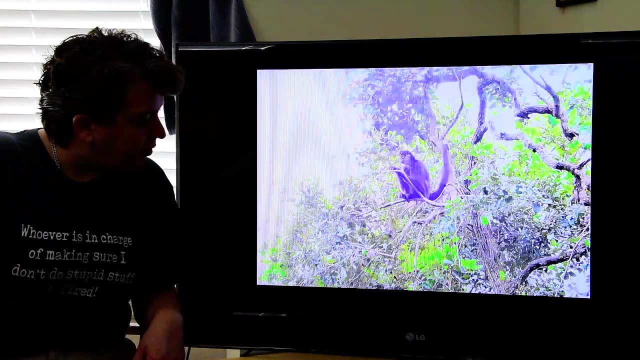 can hold onto things with their tail. This is an early branch. that is not a part of human evolution. They are kind of on their own. They are not dealing with evolution of homo sapiens. Good examples of these are things like spider monkeys and capuchin monkeys. 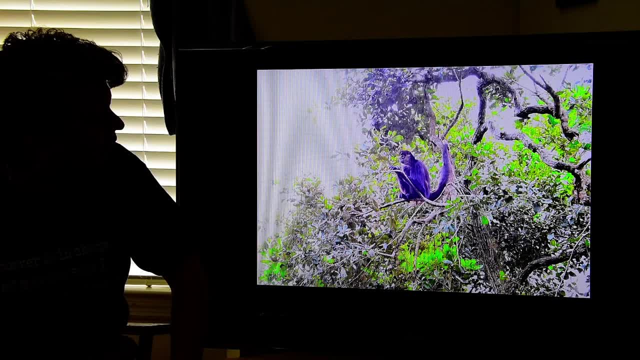 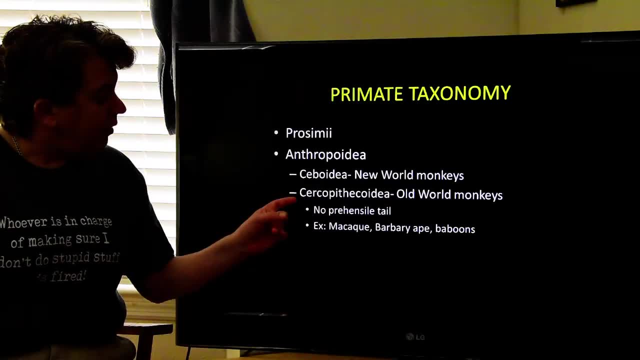 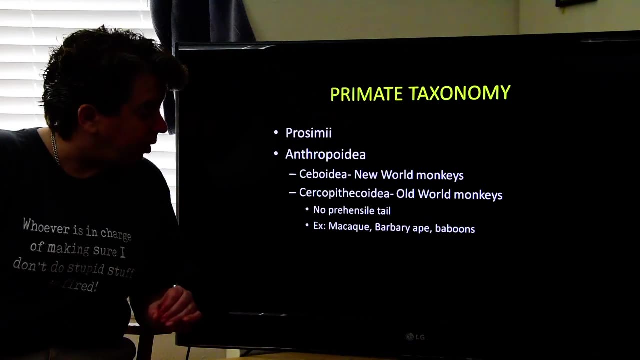 That is a monkey. I don't know exactly what kind, but I took a picture of it in Belize. So that is a new world monkey. We also in the anthropoidea group we have cercopithecoidea. These are old world monkeys. 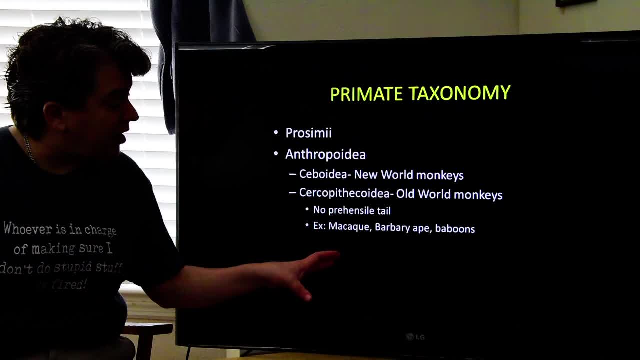 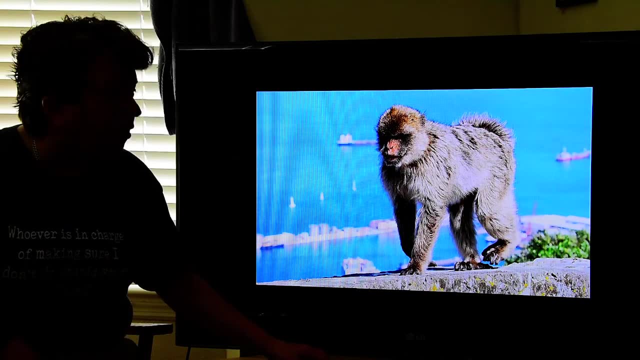 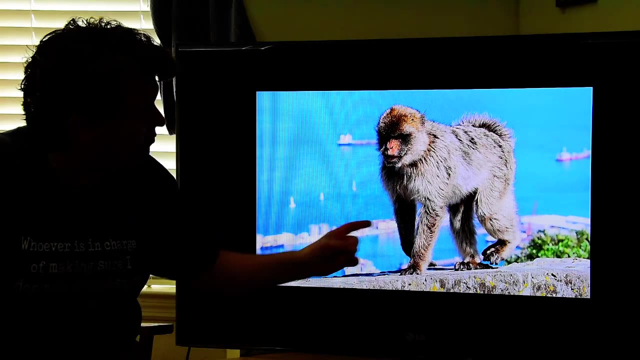 They do not have a prehensile tail. Some examples are macaques, Barbary apes and baboons. This is an old world monkey. This is off on the Isle of Gibraltar or Rock of Gibraltar. There is an interesting story about these. 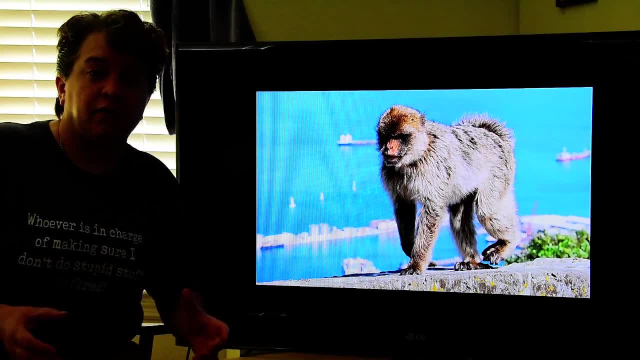 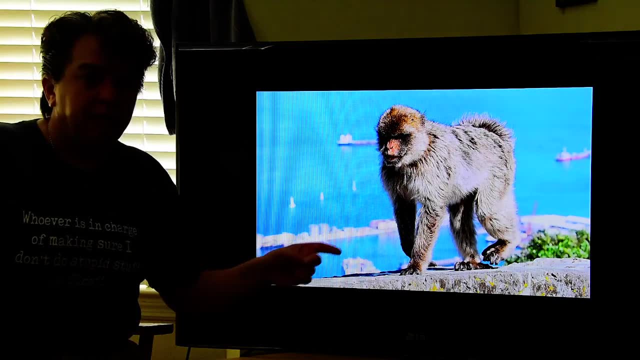 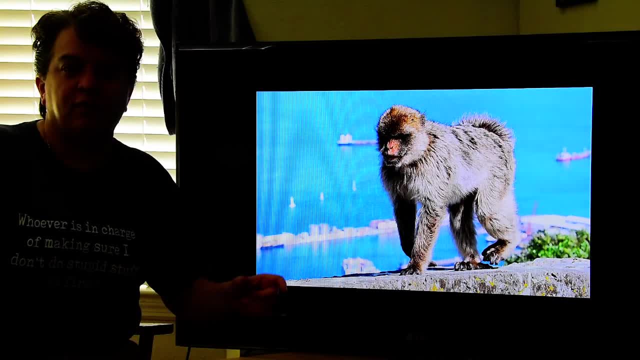 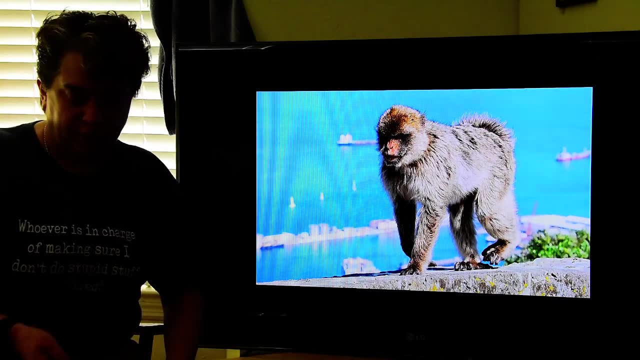 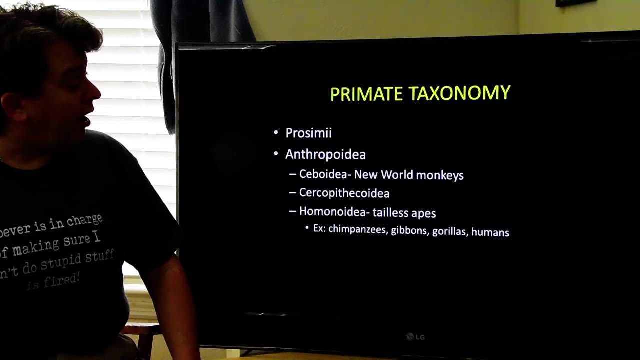 They were very aggressive. The bad monkeys were rounded up and they were exiled to Scotland where they live on some game refuge or something and don't have any tourists that they can harass. So this is one of the ones that I think got exiled to Scotland. 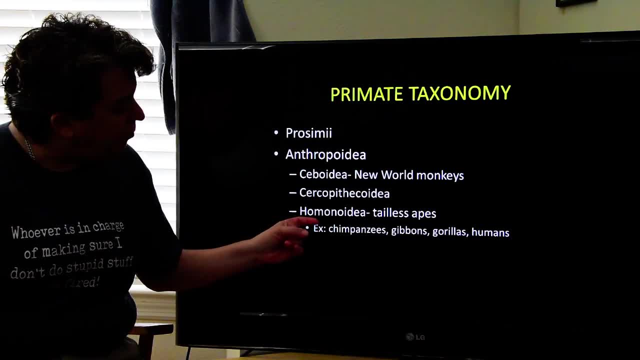 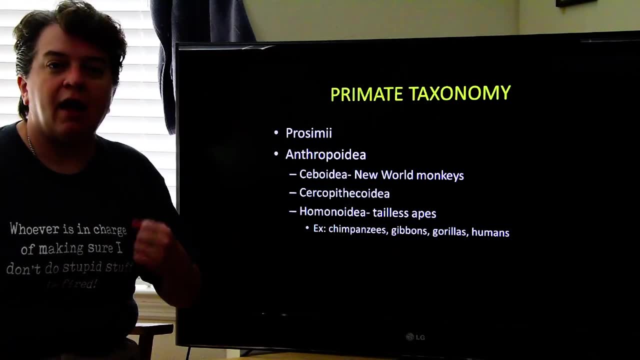 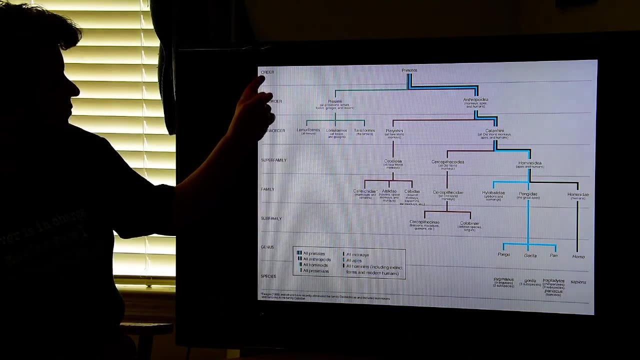 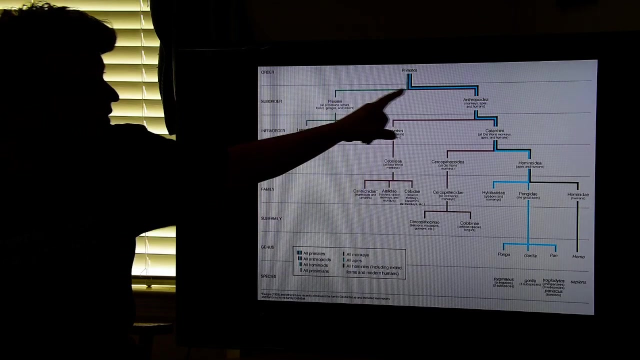 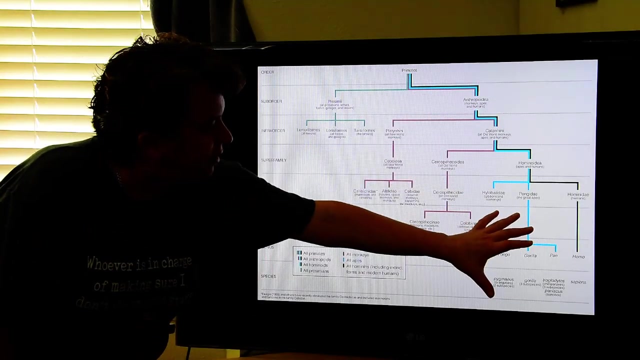 The ones that we are going to be concerned with today are Homo Noidea. These are completely tailless apes. We are looking at chimpanzees, gibbons, gorillas and humans. They are nothing but monsters. So here's our basically family tree of primates. So we have order primates there. There's the prosimi, the lemurs and stuff. There's anthropoidea. Here's the new world monkey branch. This is the branch going all the way to humans. 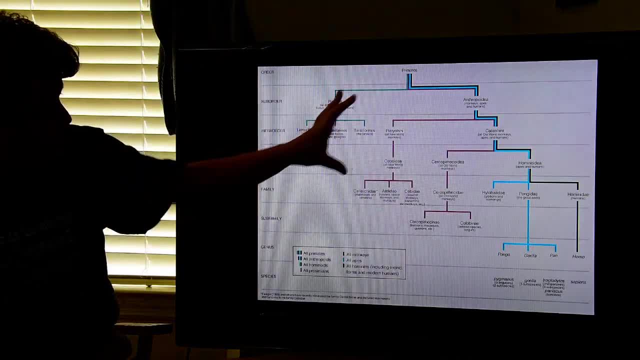 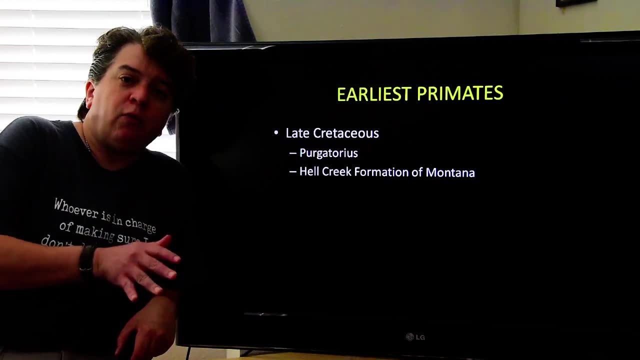 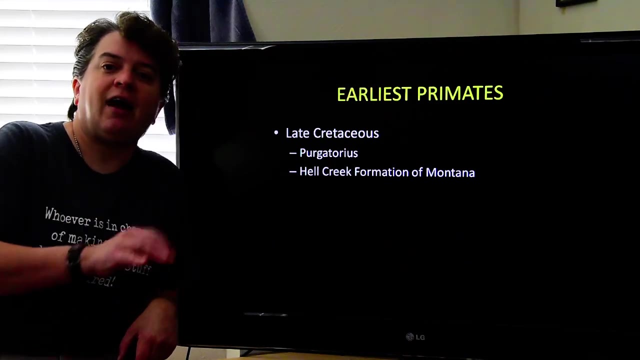 And there's the old world monkey branch, And so that's the family tree there for primates. The earliest primates actually date all the way back to the late Cretaceous, So the earliest primates were around at the time of the last dinosaurs. 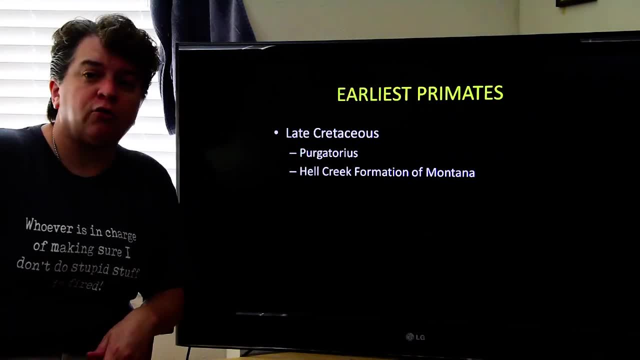 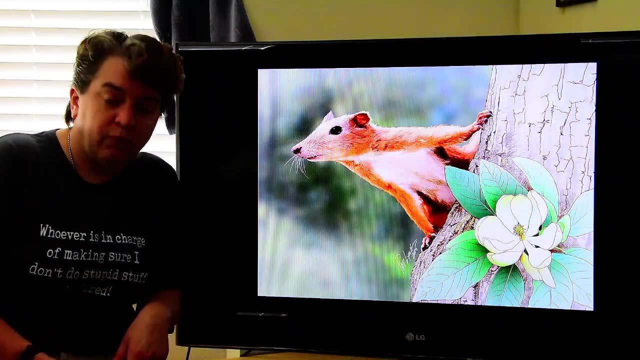 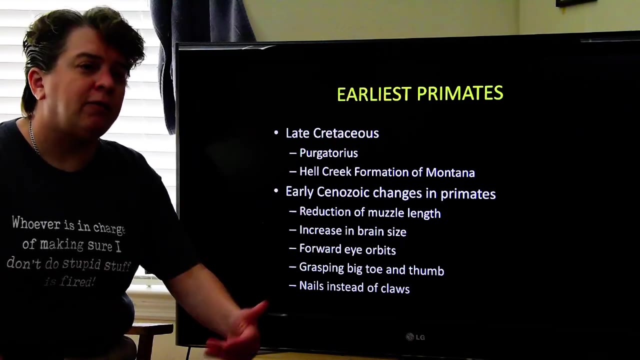 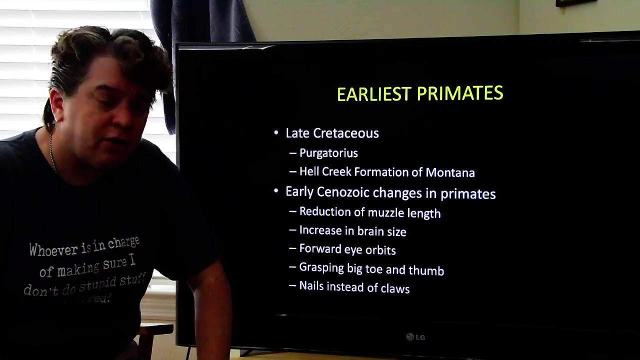 And the oldest one that we know of is named Purgatorius and is found in the Hell Creek formation of Montana. And this is what Purgatorius would look like Now in the Cenozoic. when we get to the early Cenozoic, following the mass extinction of the dinosaurs at the end of the Cretaceous, we see a number of changes occur in primates. 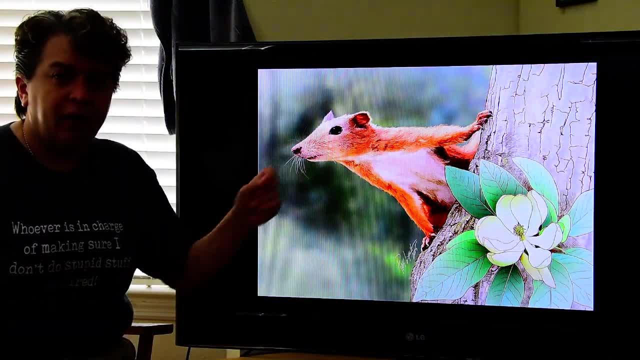 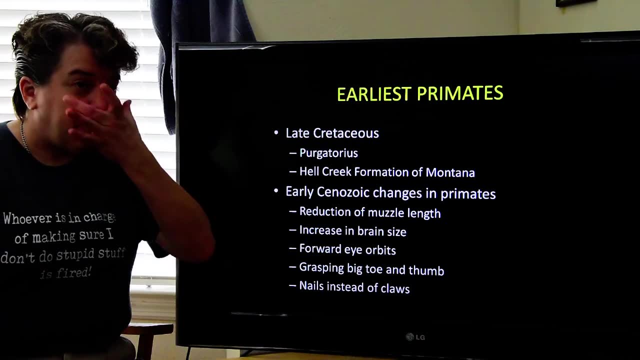 So the muzzle length right, this snout on there that starts getting shorter. We also see the brain size getting larger. Eye orbits move to being very small. Eye orbits move to being very small. The skull is very much in the front of the skull. 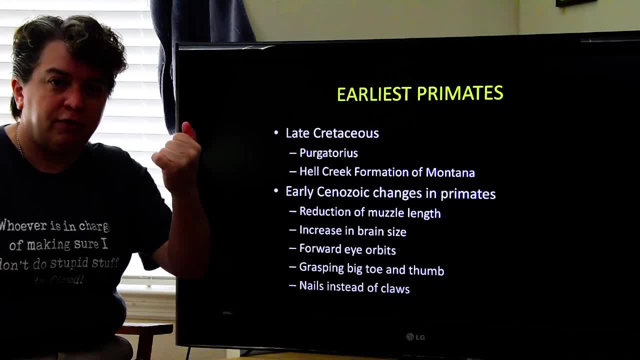 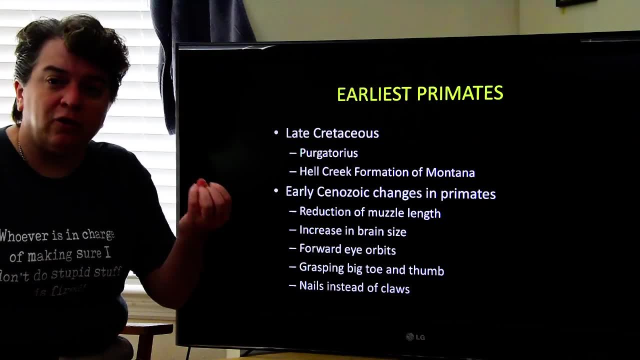 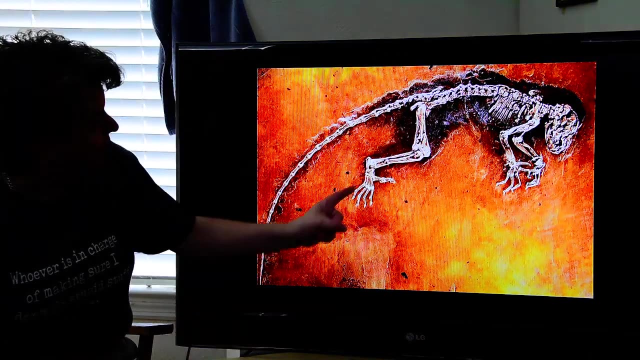 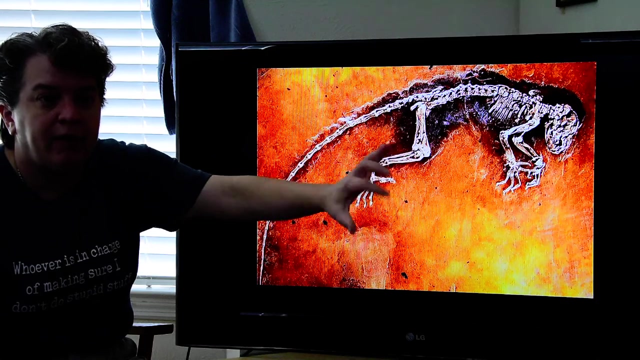 We see both the thumb for grasping and a big toe for grasping And you get nails instead of the really, really sharp claws. And this is an early primate And we can see that grasping big toe there And we can see it has hands that would be very deft for holding onto things. 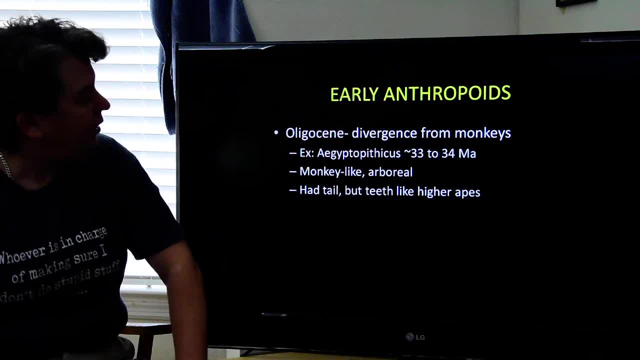 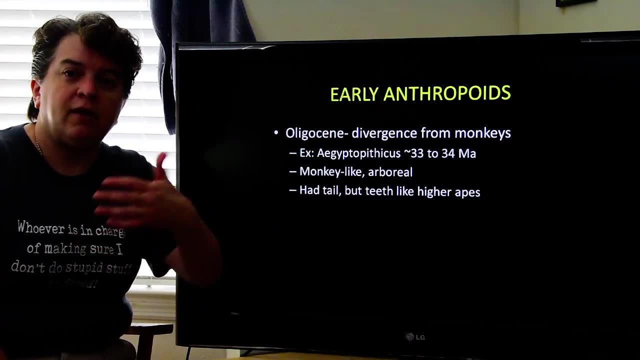 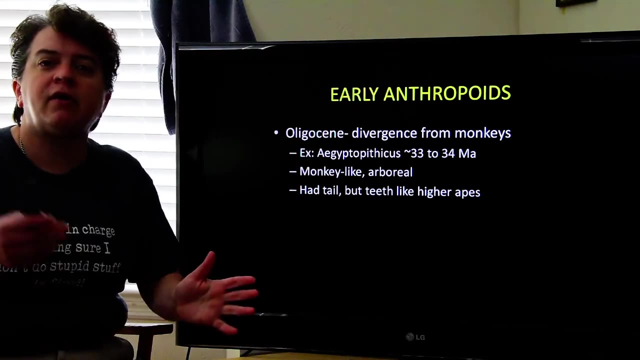 And we can see it has hands that would be very deft for holding onto things. And in the Oligocene the early anthropoids break off. They evolutionarily follow their own path away from the monkeys. So we have this divergence where the monkeys follow one path of evolution and the anthropoids follow another path. 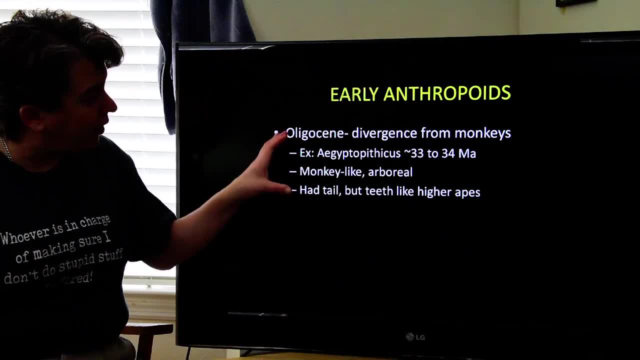 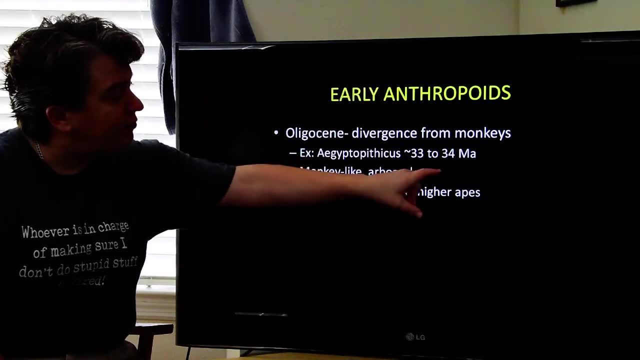 And a good example of one of these Oligocene early anthropoids is Aegyptopithecus Aegyptopithecus- Aegyptopithecus Aegyptopithecus. 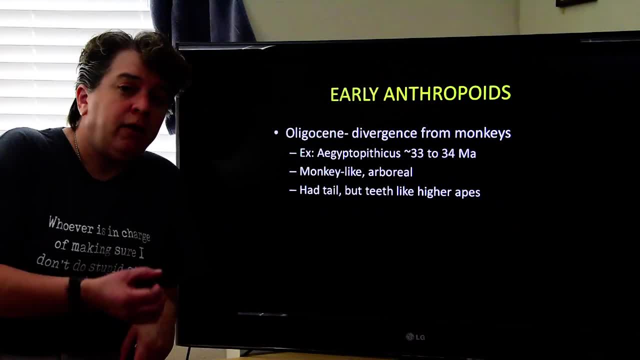 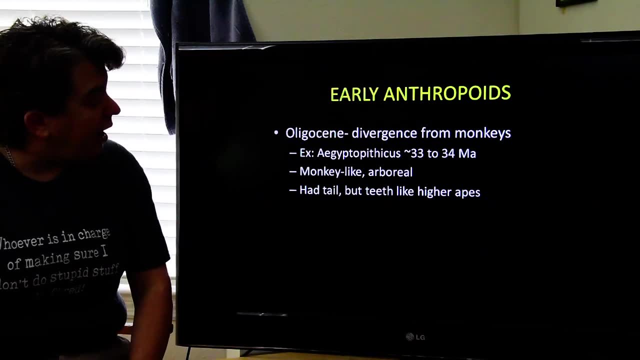 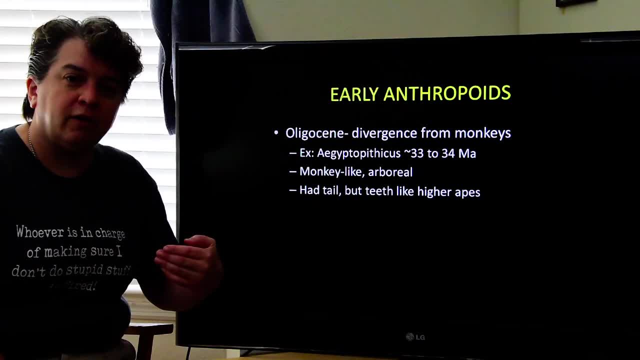 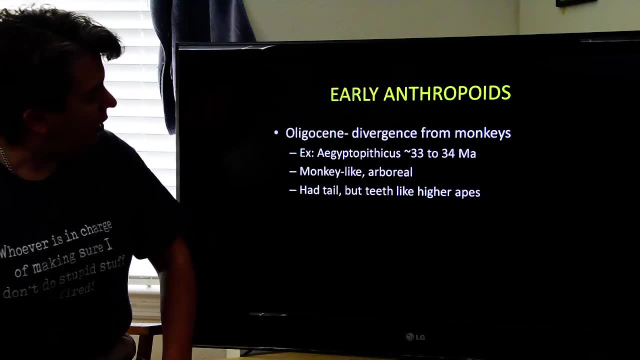 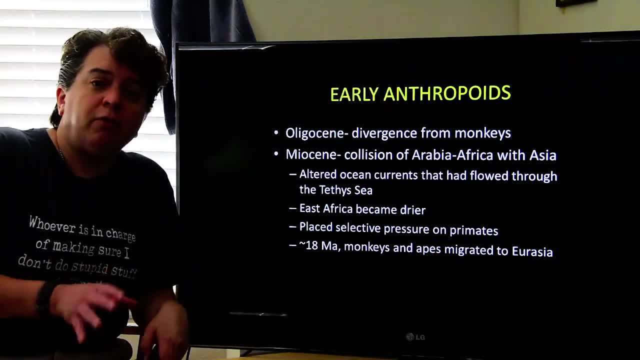 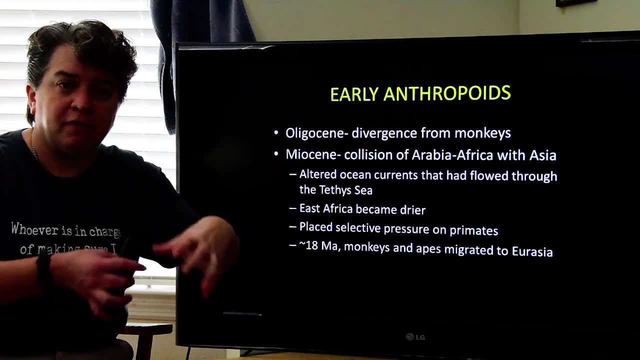 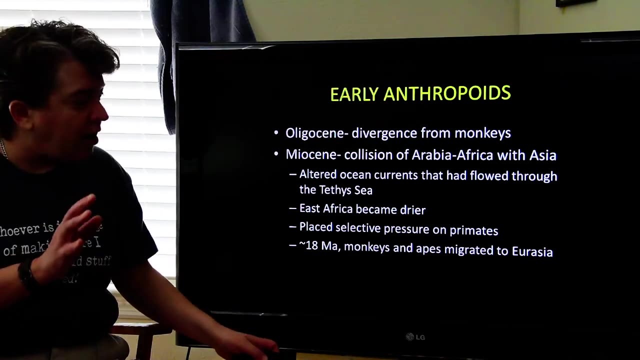 By the time we enter into the Miocene. there's a number of changes happening on Earth. At this point in time, we get Arabia-Africa, so this plate that involves Arabia and Africa collides with Asia. What this does then? it alters the ocean currents that were flowing through the Tethys Sea. 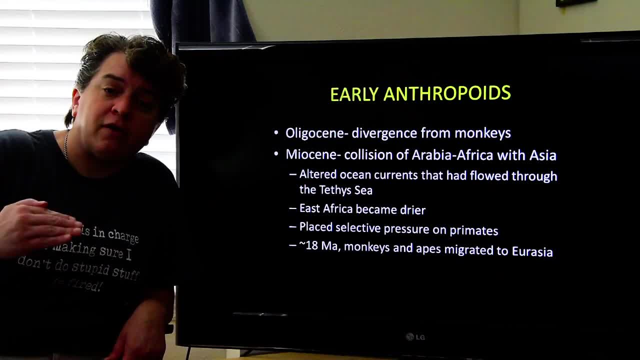 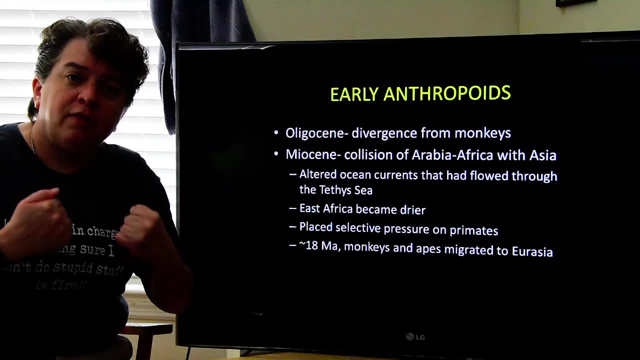 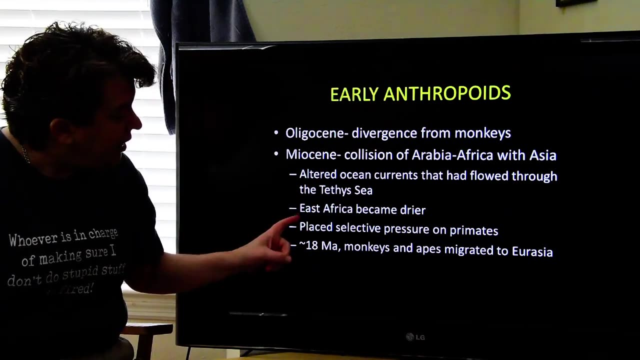 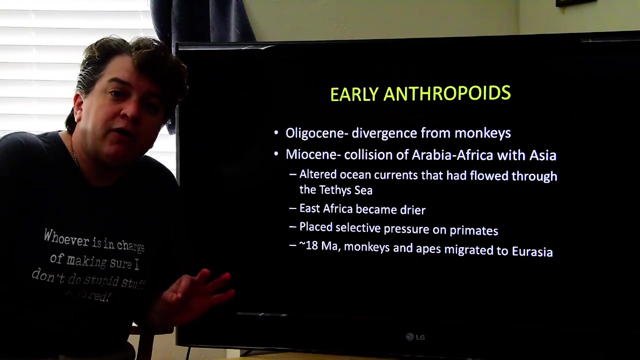 Remember that whole Tethys Sea that basically separated all the southern continents from the northern continents in the Cretaceous. We're closing that, so we're changing these ocean current patterns, which is going to change the climate system. East Africa, where our anthropoids are evolving, starts getting much drier. 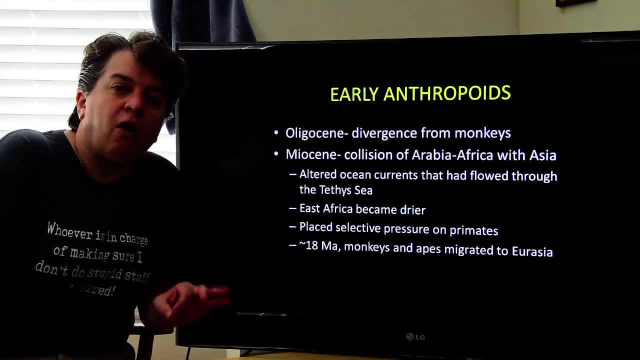 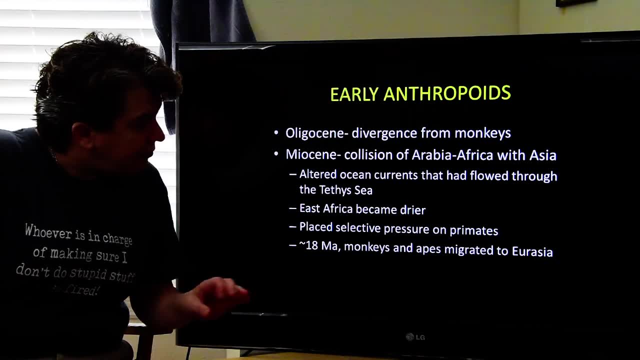 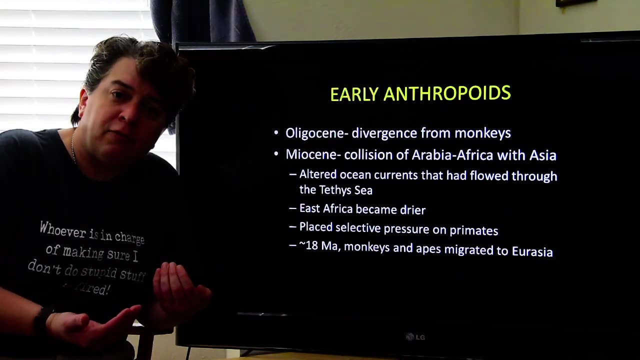 This is going to place some selective pressures on primates And this is going to change the climate system. So what we're going to see is, as things get drier, the vegetation is going to change in Africa, And that's going to mean that, just like with the horse, as the vegetation changed, 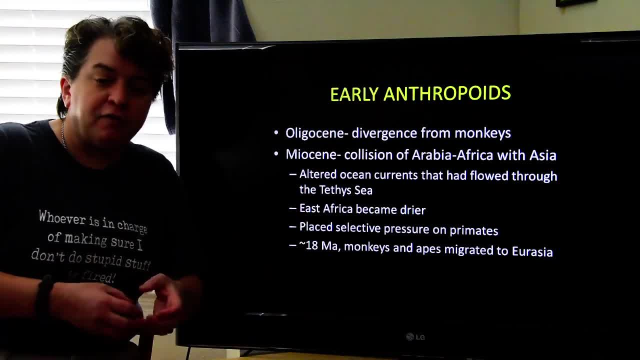 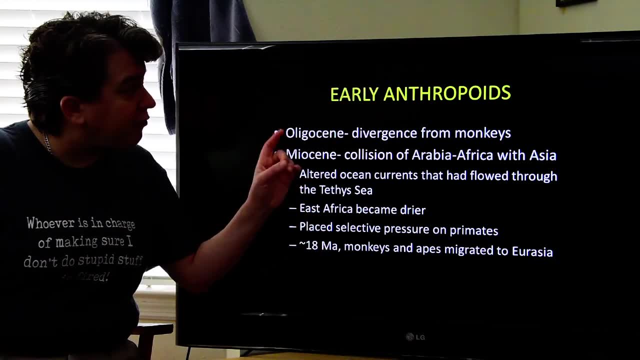 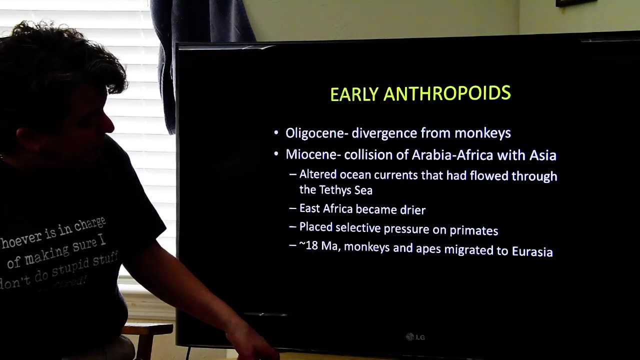 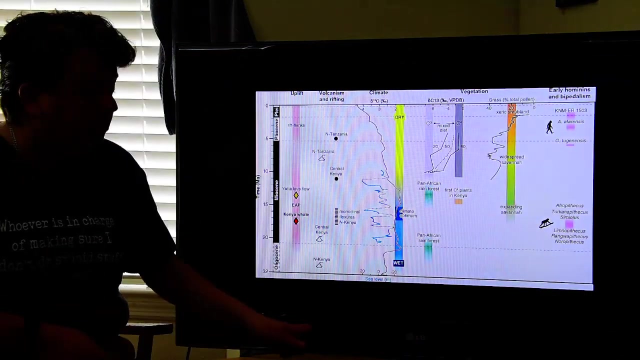 the horse had to evolve to still thrive in that changing environment. we see the same thing happen with these anthropoids. They have to change to adapt to this climate And by about 18 million years ago, monkeys and apes migrated from Africa into Eurasia. 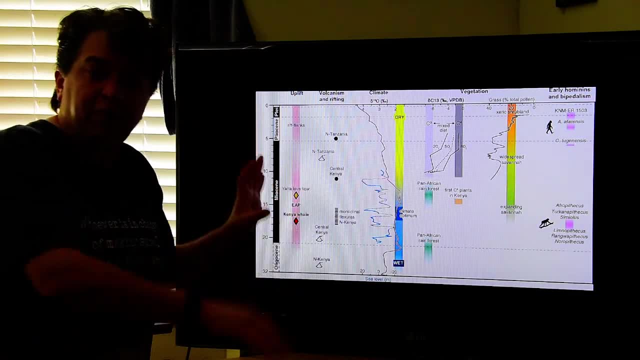 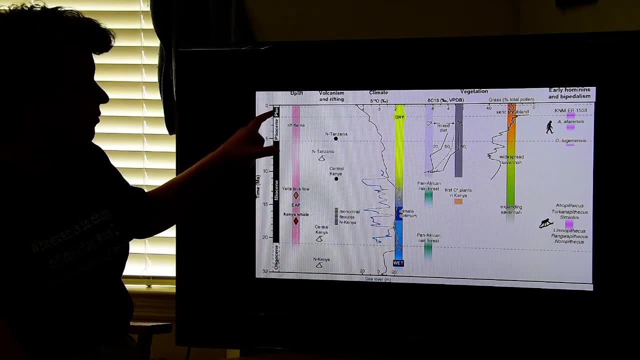 And this is what happened. I know a very busy graph, but there's a lot of very good information on here. So here we have our time periods: Oligocene, Miocene, Pliocene, Pleistocene, and then that's. 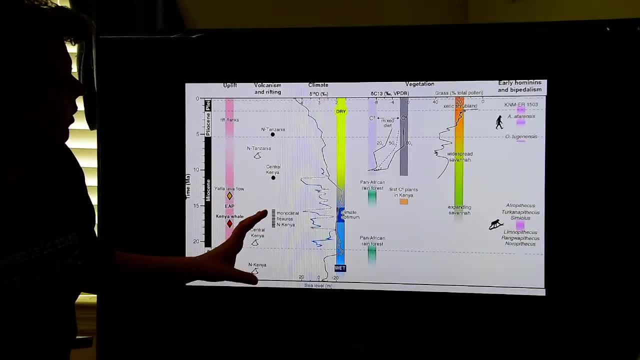 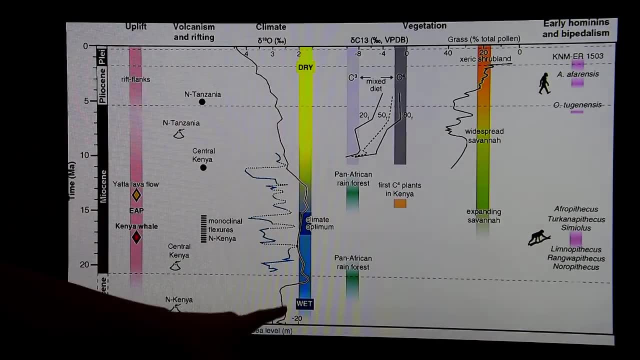 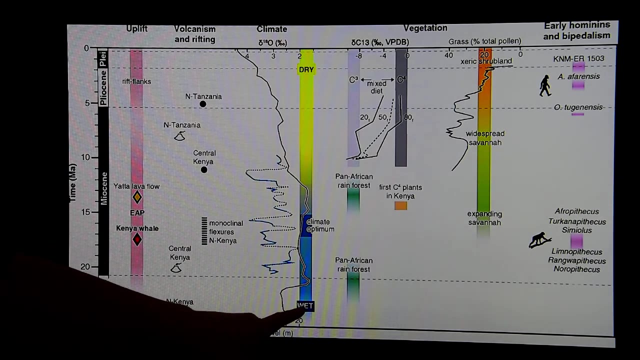 the Holocene right there Now. things I want to point out that are important in here is, for example, this: This is the climate, And what we're looking at is back here. The climate in East Africa. East Africa is wetter and as we progress closer to the modern day, it gets drier and 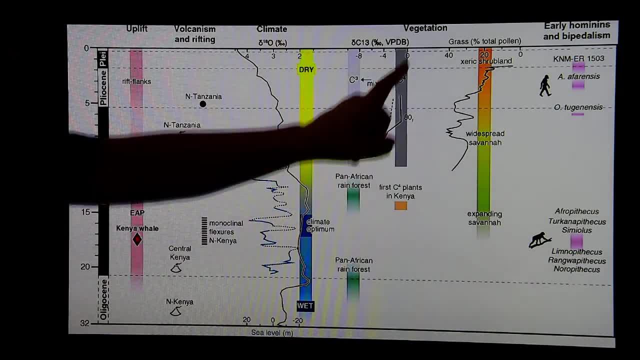 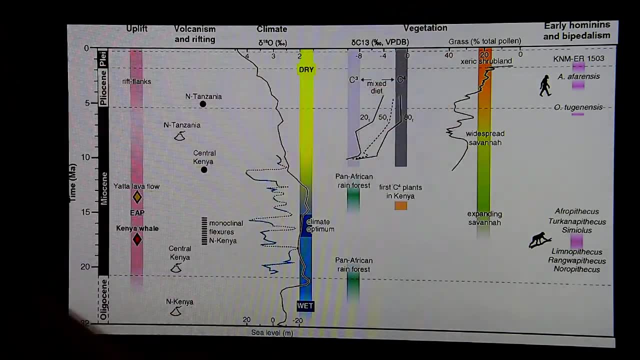 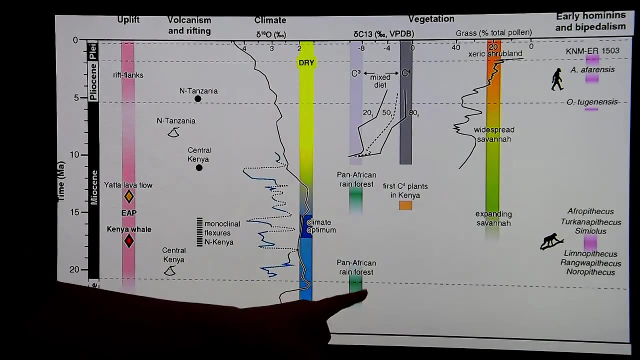 drier And that's then going to affect the vegetation. So here are some graphs concerning vegetation And you can see here we had a rainforest right. Pan-African, that means all across Africa- we had this rainforest. 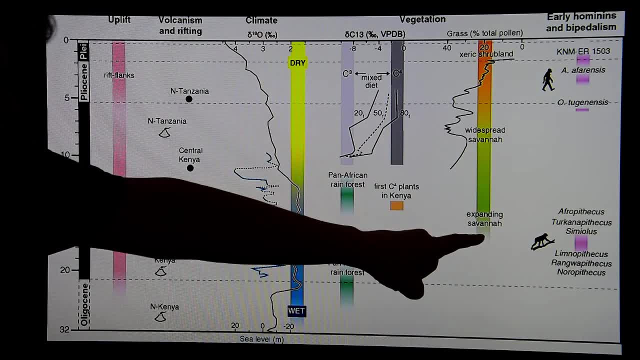 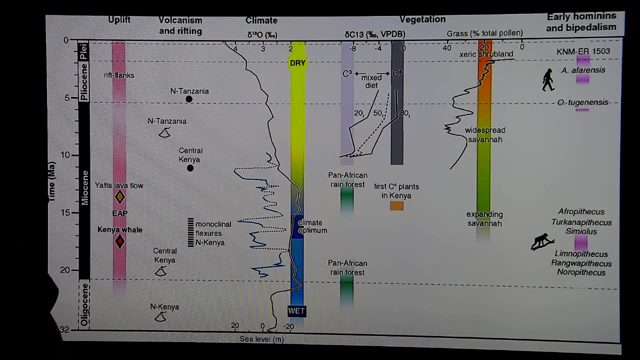 But we start seeing it going away and we start seeing the savanna expanding More savanna. And a savanna is a grassland with a few trees. It's very much like kind of our prairies here, except you have a few trees dotting that area. 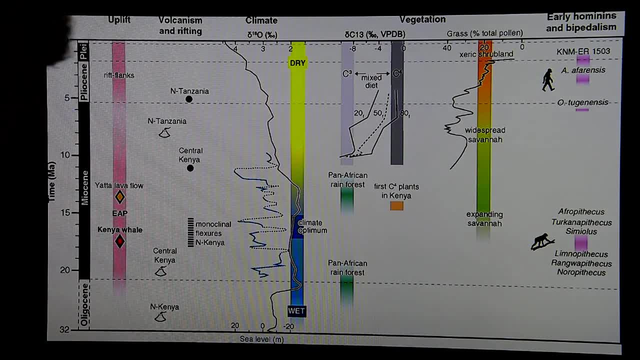 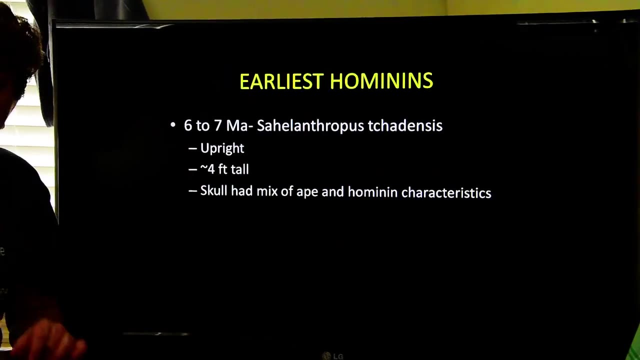 So what we're seeing, then, is this change from having lots and lots of trees right That rainforest to having lots and lots of grassland, And that is going to impact the climate, And that is going to affect the climate And that is going to affect the evolution of the hominids of our group. 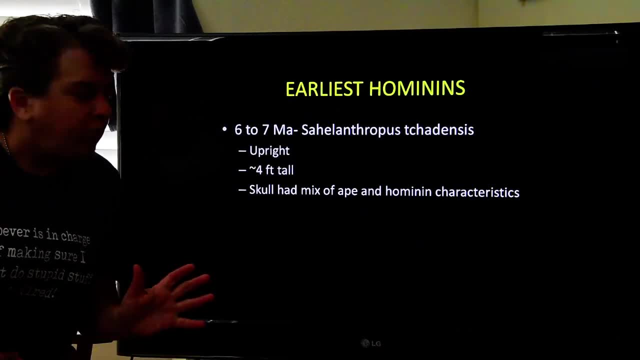 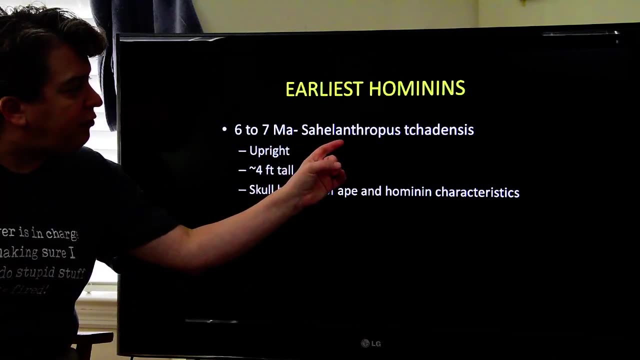 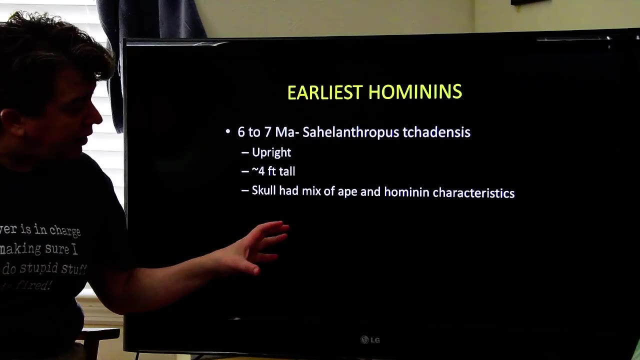 So let's look at our earliest hominids and we're going to go to about six to seven million years ago, And we have Sahelanthropus chadensis. He's upright and he stands about four feet tall and the skull, if you look at it, has. 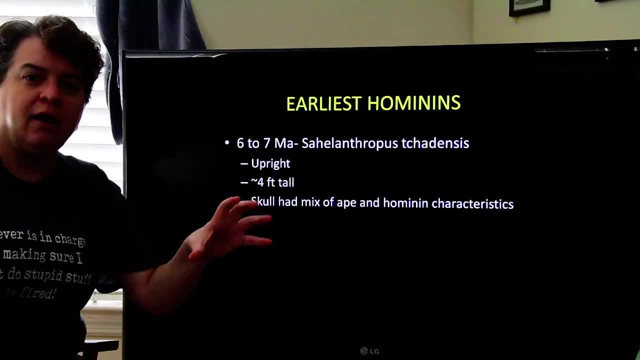 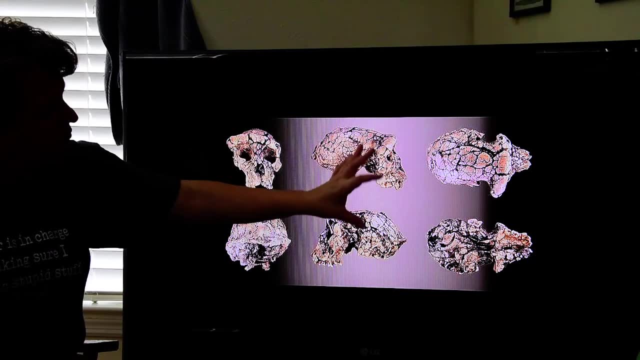 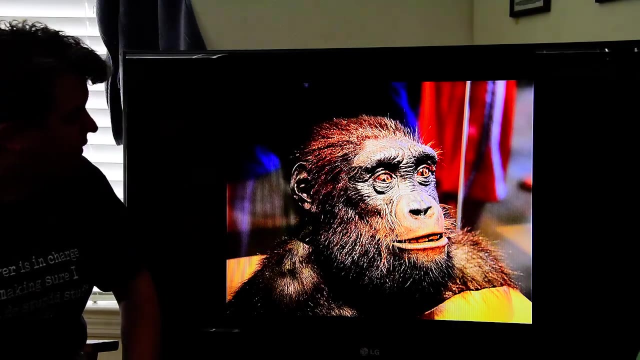 a mix of both kind of ape features and morphology, More hominin features, And we can see this skull right here. right, it does have a lot of ape-like features, like some of these brow ridges and things, But notice that we're getting a larger brain case, something very typical of later hominids. 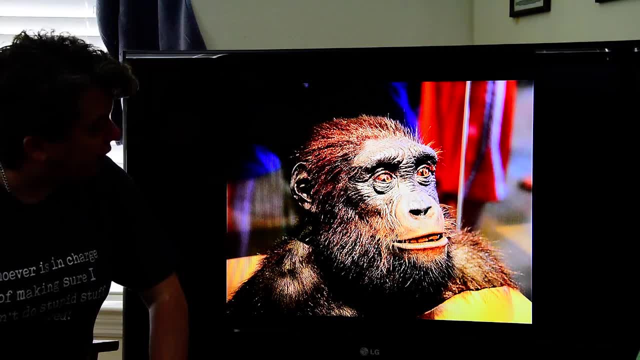 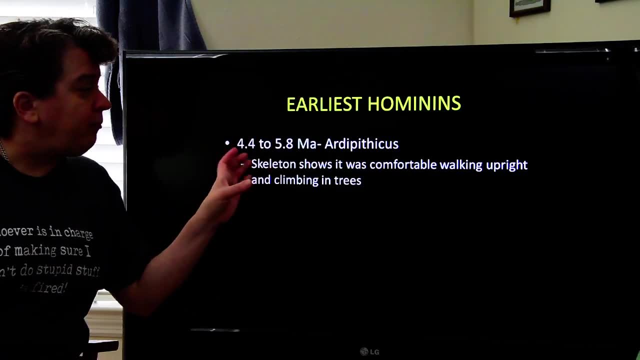 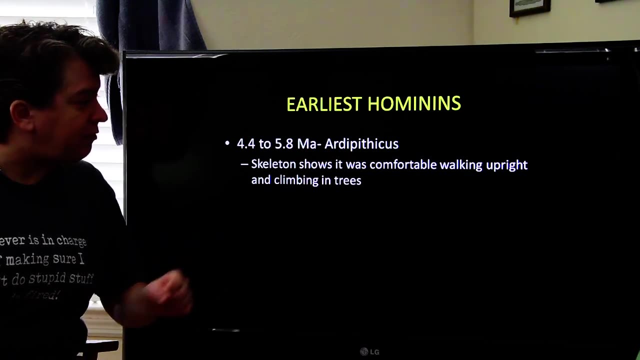 But this is what that organism probably looked like. that's, you know, our best estimate. Now we're going to move forward a little bit and we're at about 4.4 to 5.8 million years ago. We have Ardipithecus. 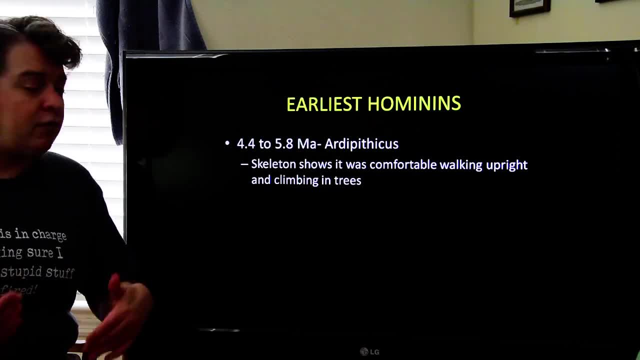 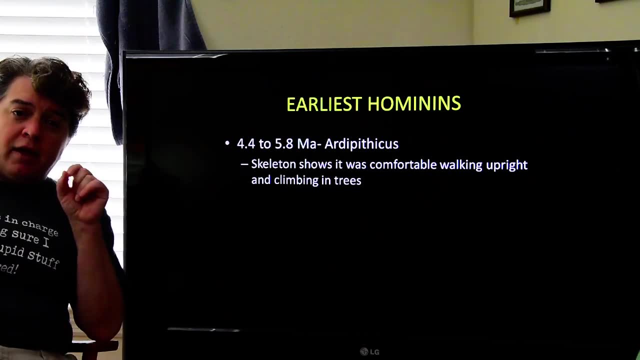 And the skeleton, when we look at Ardipithecus, shows that it was comfortable both walking upright and climbing in trees. Now remember what I was saying about the climate. right, We had a lot of trees to begin with, but then we're starting to get more and more grasslands. 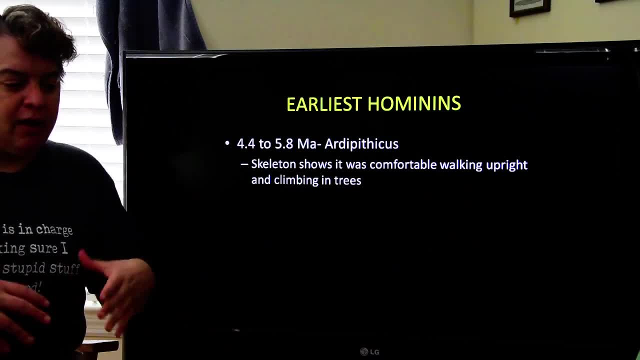 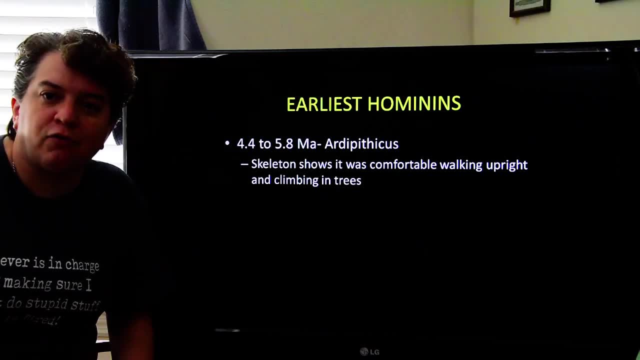 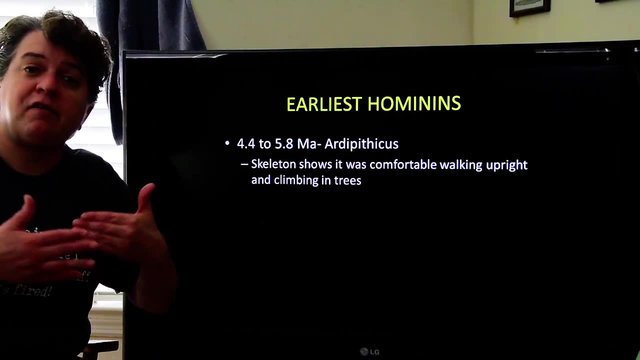 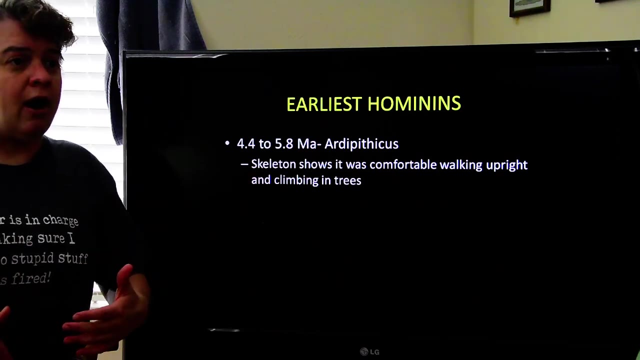 They have to adapt to not having as many trees to travel in and trees to hide from predators in and things like that, and have to now survive in these expanding grasslands. And how to do that? Standing straighter, standing taller, walking bipedally, walking upright. 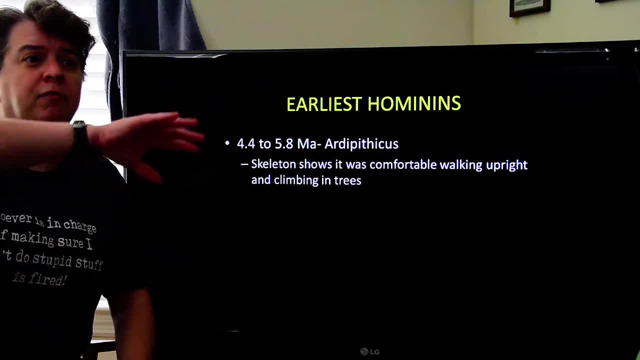 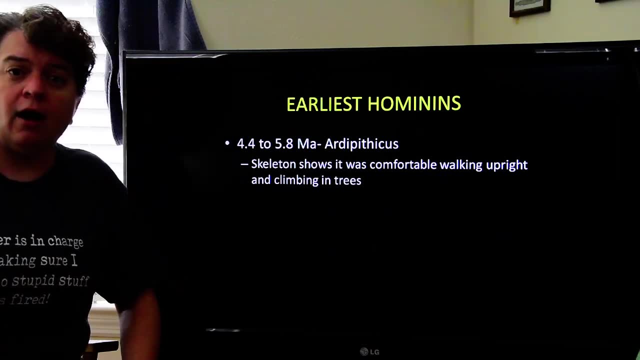 What does that give you an advantage? Well, you can now see above the grasses. You can see predators that might be coming. You can move relatively. You can move relatively quickly on the ground if you can't get into the trees to hide from. 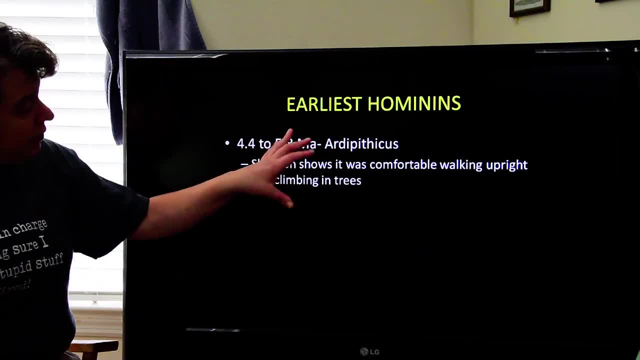 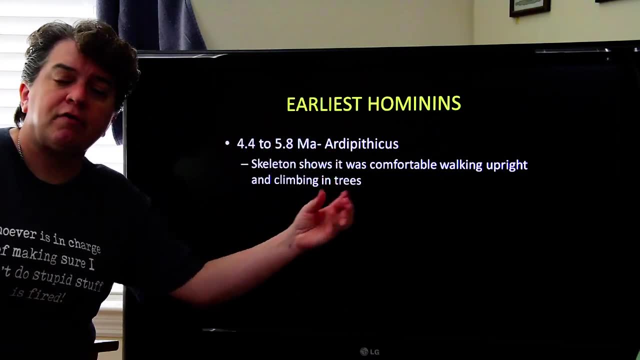 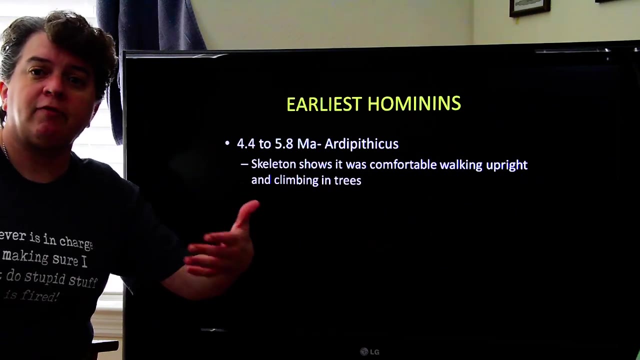 predators. And so we're kind of having this moment here where it both still kind of carries over some of the arboreal characteristics of the earlier organisms, but we're also moving to that more modern and having to deal with living in these drier grasslands. 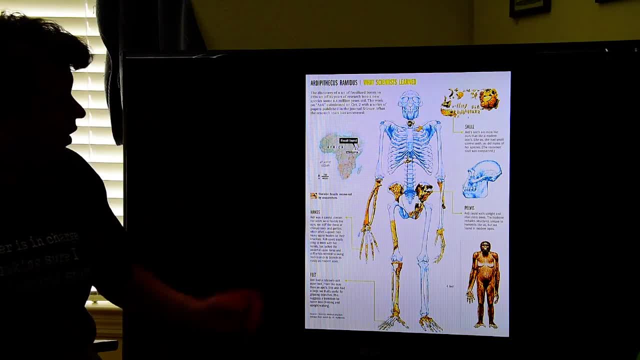 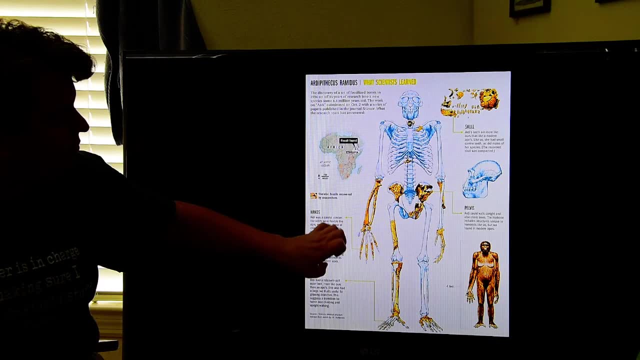 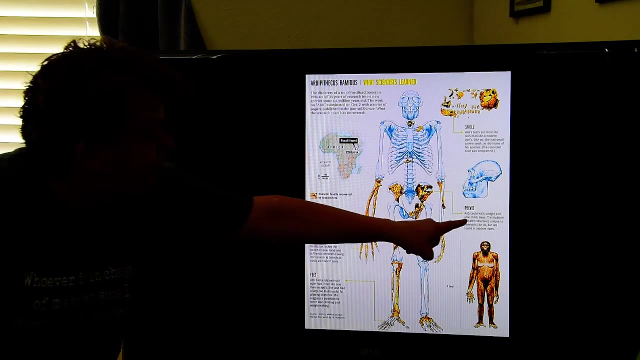 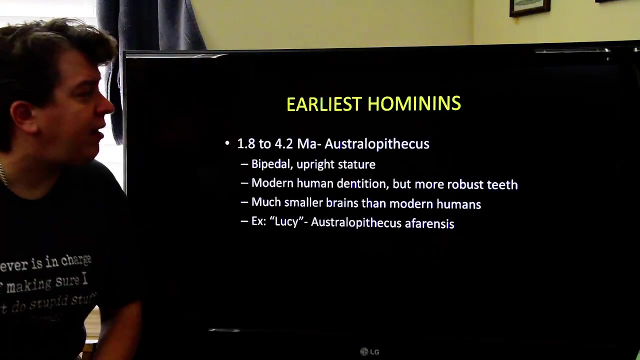 So this is some of the skeleton of the hominid. This is a little bit more of a, And you can see it still has these very long arms that are typical for climbing, But it also- the pelvis- shows that it could walk upright. 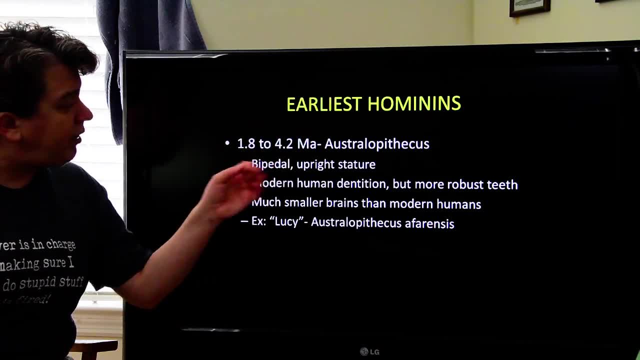 Now let's go to Australopithecus, which is a relatively famous of this early hominids. 1.8 to 4.2 million years ago This was bipedally. Now you can see that this is a very long arm. 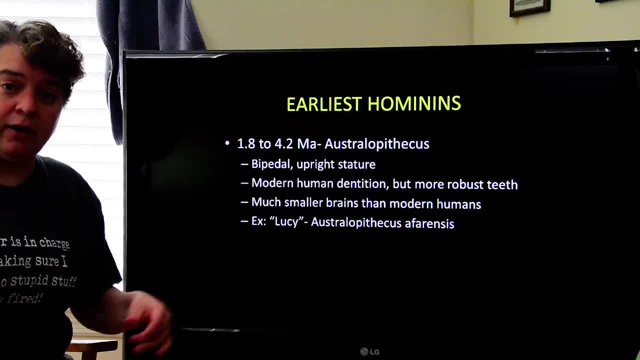 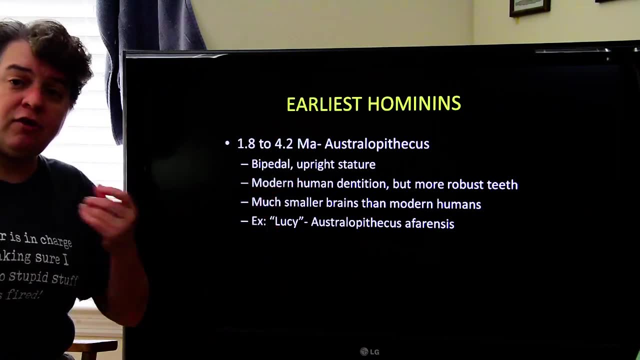 And it's very, very long And it's very, very short And it's very, very short And it's bipedal. So Australopithecines walked on two legs, had this upright stature, The dentition, the teeth looked very similar to modern humans, but they were more robust. 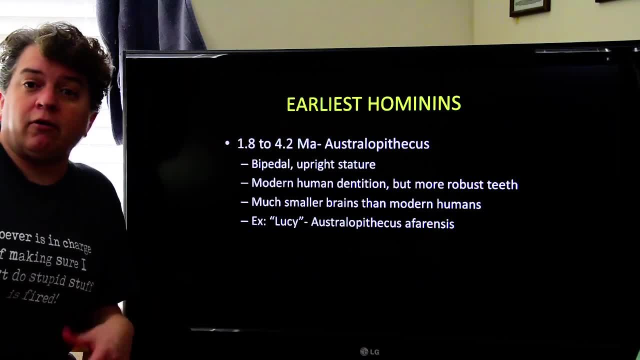 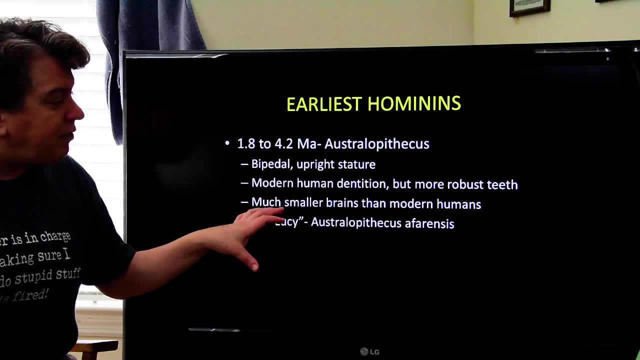 They were kind of stronger probably for- you know, I don't know- cracking open nuts, eating them, something like that. So kind of similar to our teeth, but just beefier. Now they do, while their brains were bigger than earlier primates. 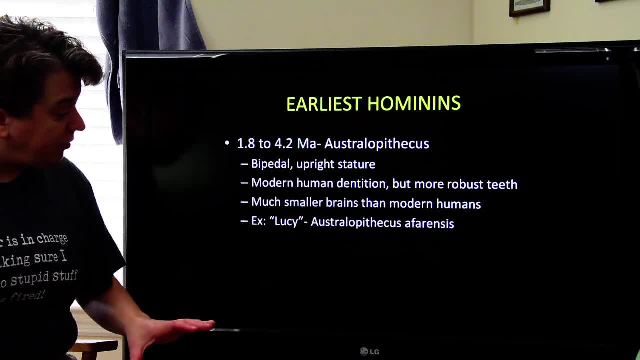 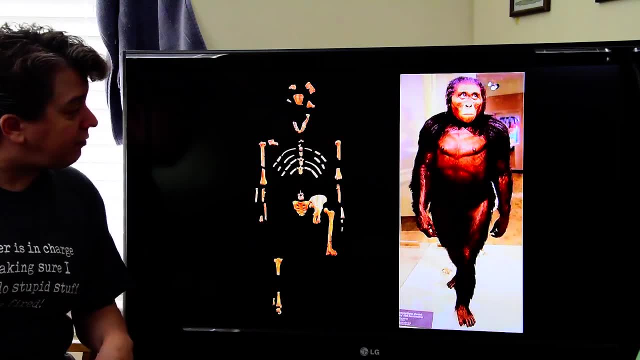 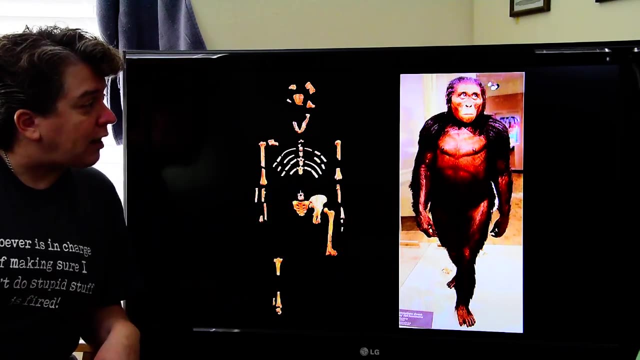 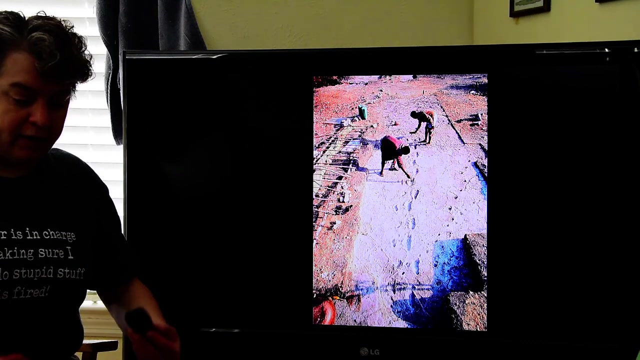 They are smaller than what modern humans have. And Lucy, the very famous fossil, is Australopithecus afarensis, And this is the Lucy skeleton And this is a reconstruction of what she probably looked like. Now we do know how these Australopithecines walked and what kind of, what kind of stride. 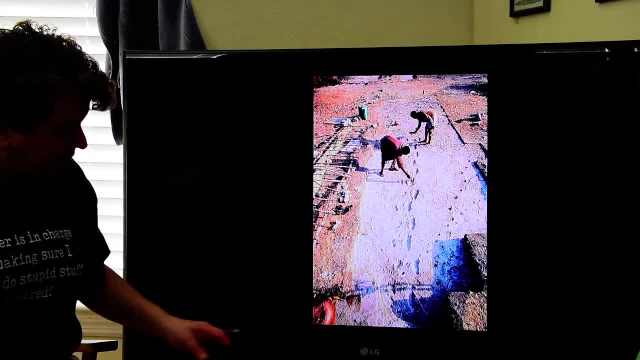 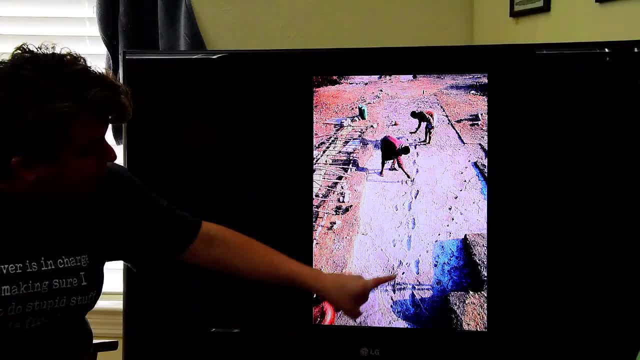 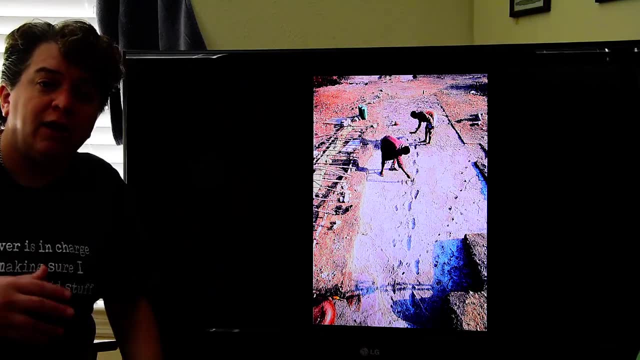 Not long after nearly 1850, this trackway, these footprints have been excavated. And what happened there? There was a volcanic eruption where a bunch of ash fell and then it rained, so you had this kind of wet, muddy, ash-type stuff. 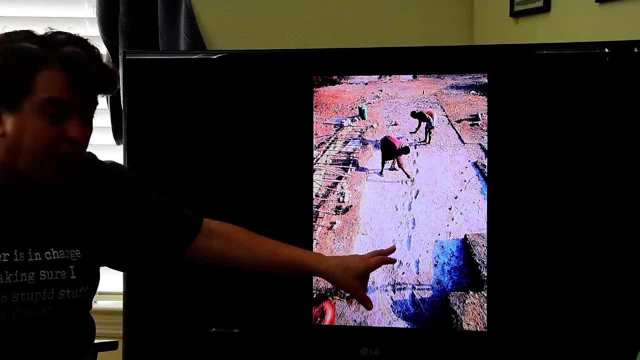 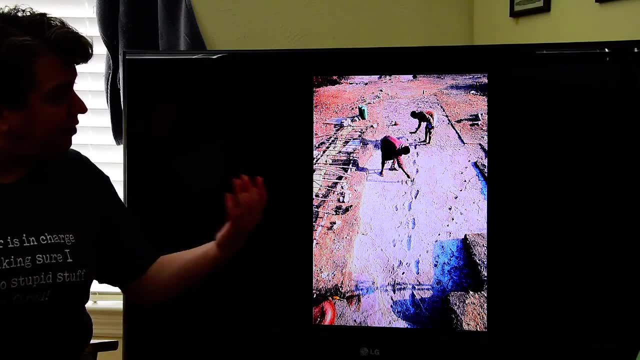 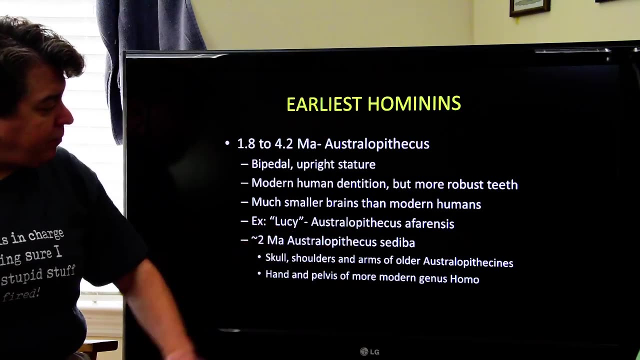 And a couple of Australopithecines- an adult and a child- walked through that area, So we can actually see what like how they walked, And we can see that they did indeed walk completely upright. Now, in addition to Australopithecus afarensis, there is another Australopithecine from about 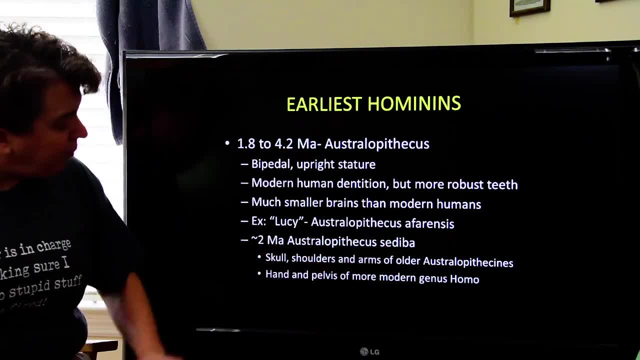 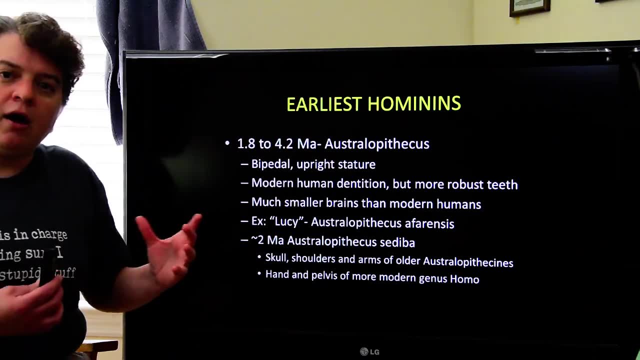 2 million years ago called Australopithecus sediba, And in this case this is kind of a mix of both older and newer hominid characteristics: The skull, the shoulders and the arms look a bit like the older ones. 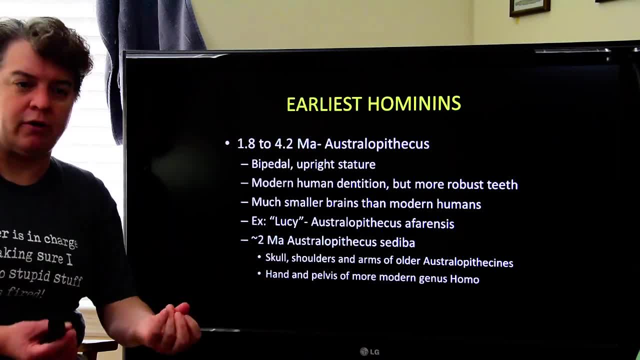 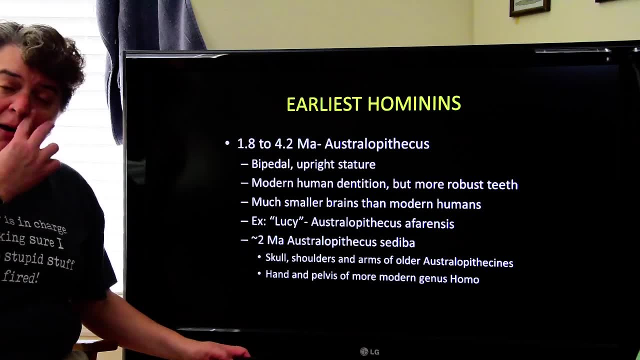 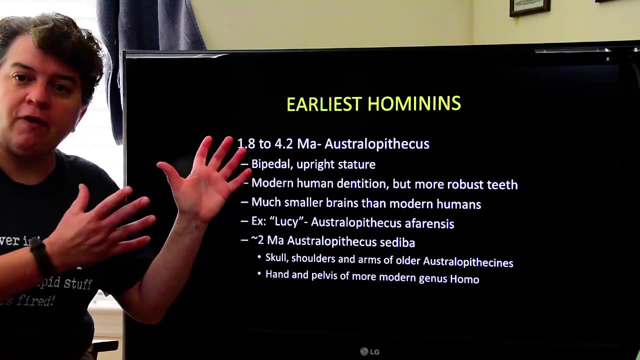 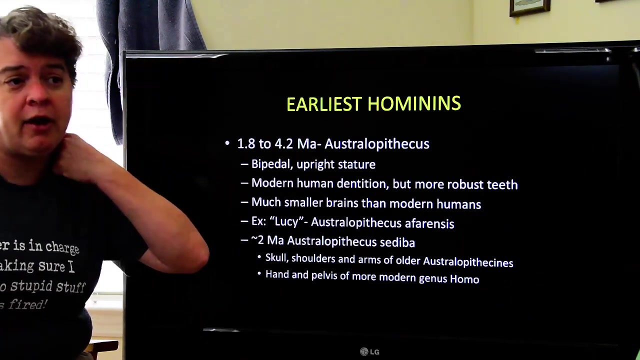 But the hand and the pelvis look a little more modern, like it could carry out some more intricate work with its hands and things. So what we're seeing at this time, as Africa is drying out and the hominids have to move out of those forests that are disappearing and move into these grasslands that are appearing. 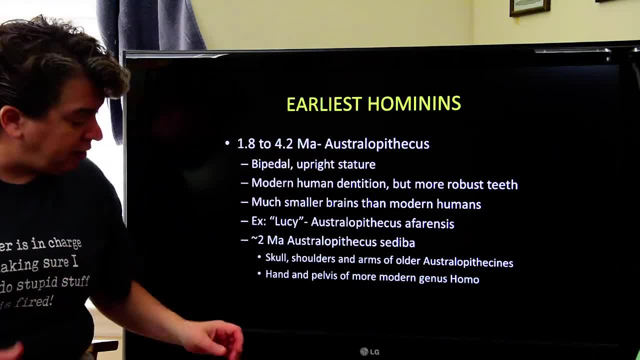 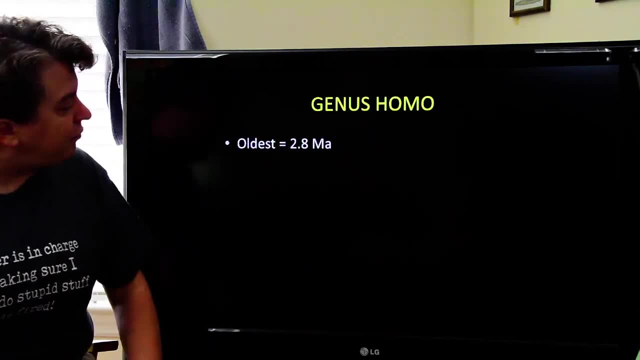 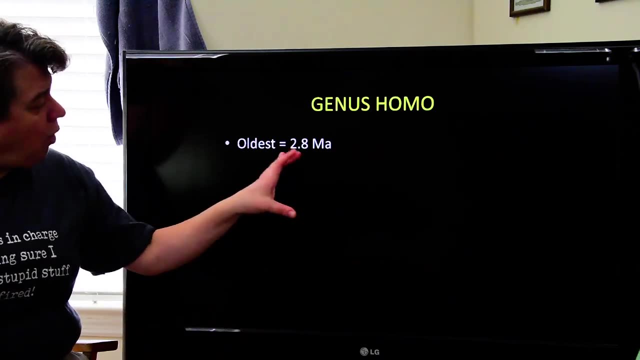 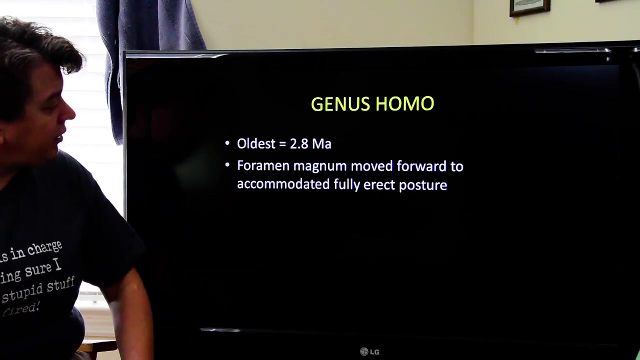 we are slowly seeing these adaptive changes. right, Natural selection is selecting for characteristics that will be better for inhabiting those savannas. Now, genus Homo. that's what we belong to, right, We are Homo sapiens, And the oldest organism that belongs to this genus dates to about 2.8 million years ago. 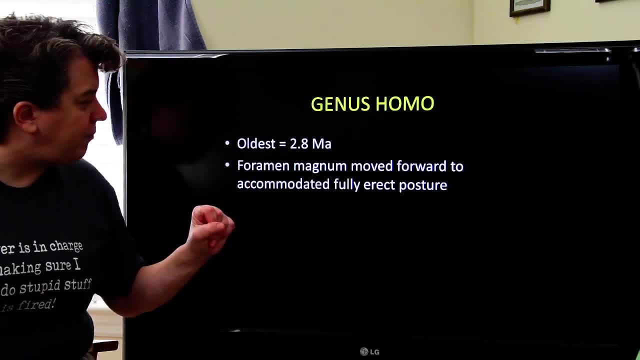 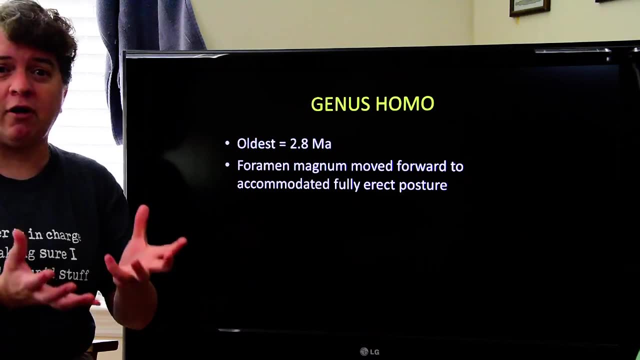 And in this genus the foramen magnum is moved forward to accommodate a completely erect posture. Now, the foramen magnum. usually I have a skull that I can hold here and show you guys. I don't, unfortunately, because I just don't happen to have a human skull sitting around. 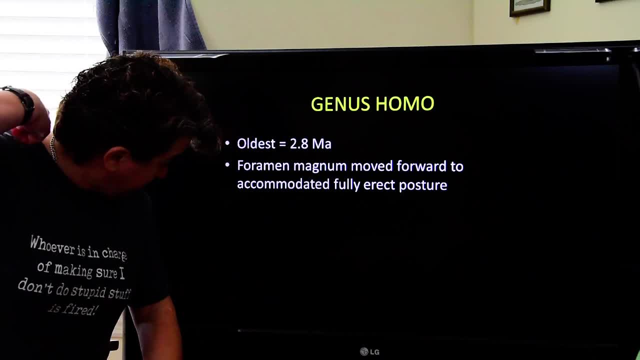 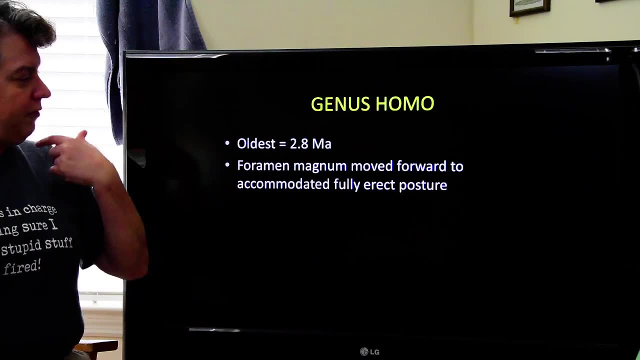 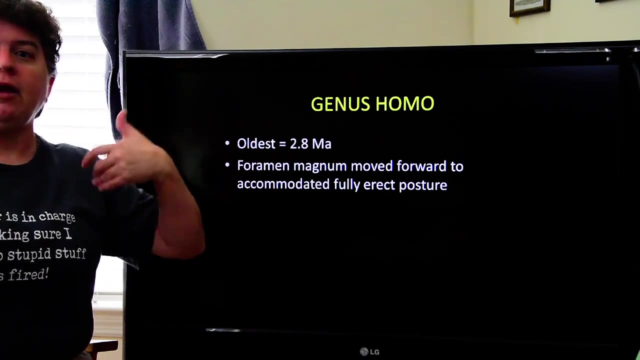 my house, But basically where your spine connects into your head, that's the foramen magnum, And it has to be kind of, instead of being at the back of the head, it kind of moved this way slowly to accommodate comfortably standing fully upright. 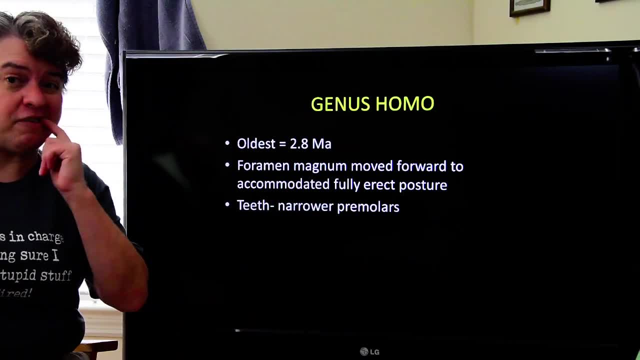 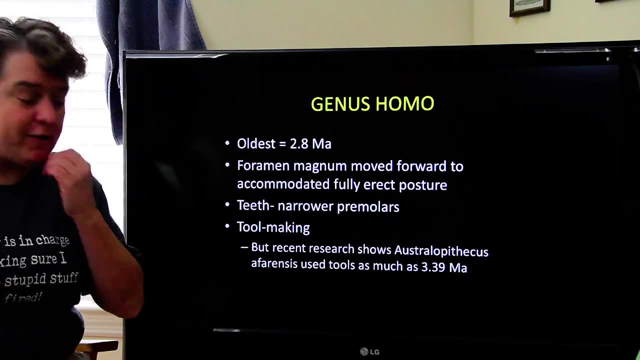 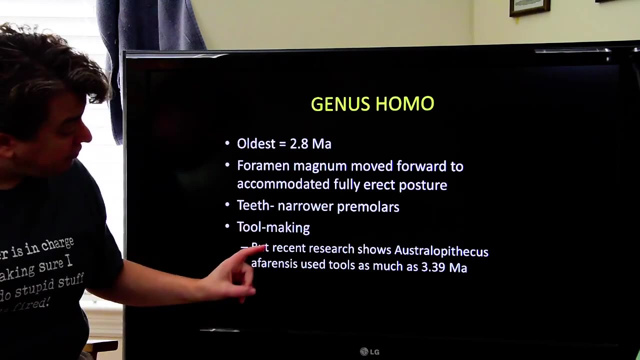 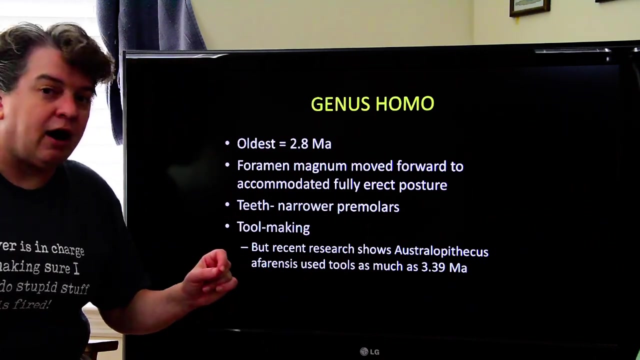 Now teeth, Our premolars get a bit narrower And tool making. Well, Homo is characterized by the fact that these organisms made and used tools. However, some recent research shows that Australopithecus afarensis actually used tools as long ago as 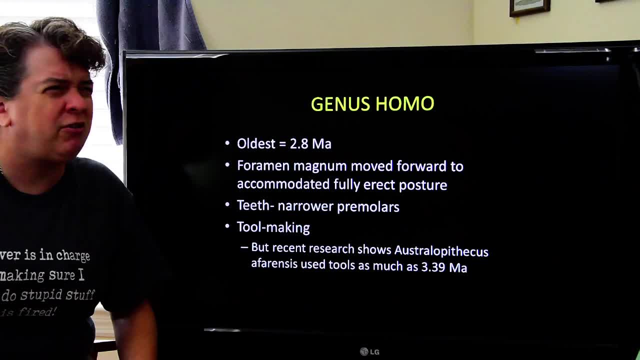 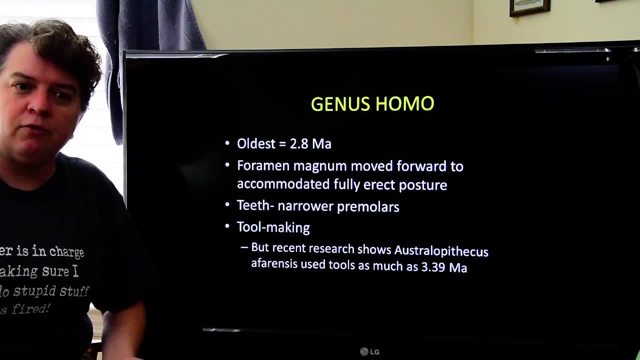 almost 3.4 million years ago. That was a paper I read just, I think, last year. Okay, And so this shows that the ability to shape tools and figure out how to use them and what the best shape would be is not unique to genus Homo. 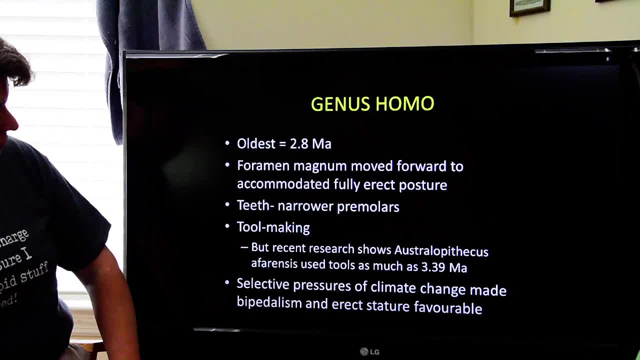 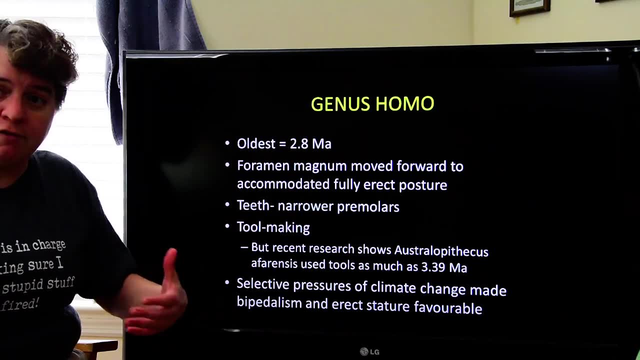 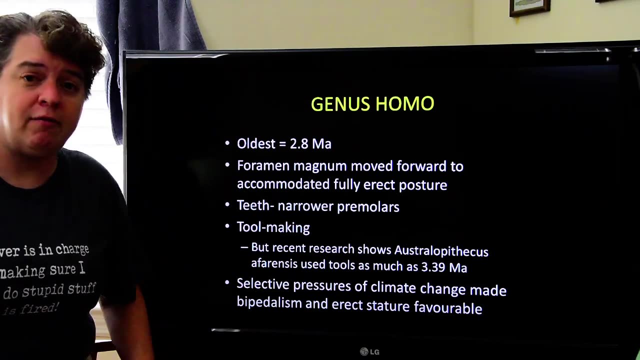 So that's kind of some interesting recent research. Now, as I said, selective pressures of the climate change, moving to those more arid grassland and savanna made bipedalism and this erect stature preferable, Because if you're not having a forest anymore to climb around in, 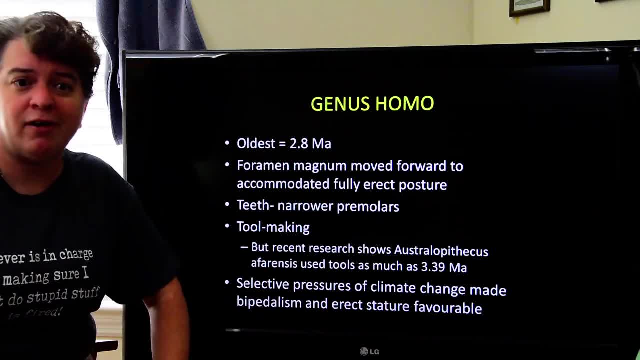 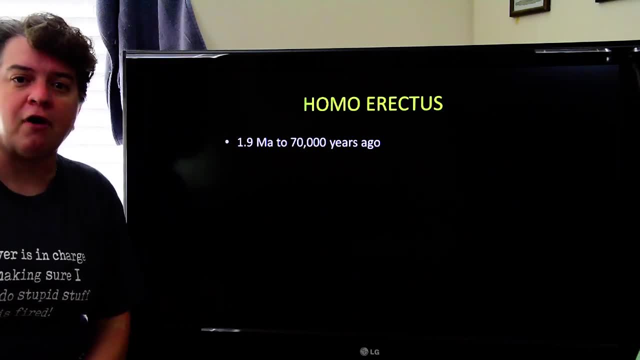 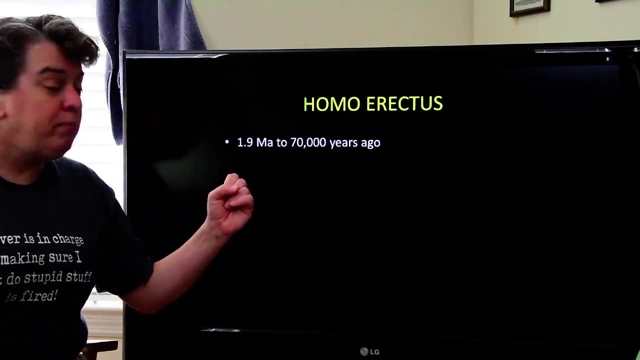 well, those characteristics of needing to climb around in trees aren't necessary anymore, right? So anyway, let's take a look at some of these early genus Homo family members. Homo erectus lived from about 1.9 million years ago to 70,000 years ago. 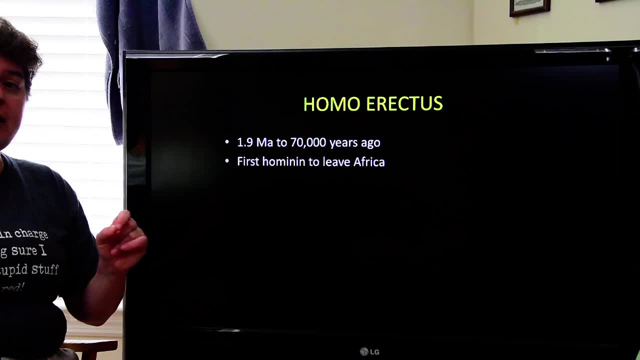 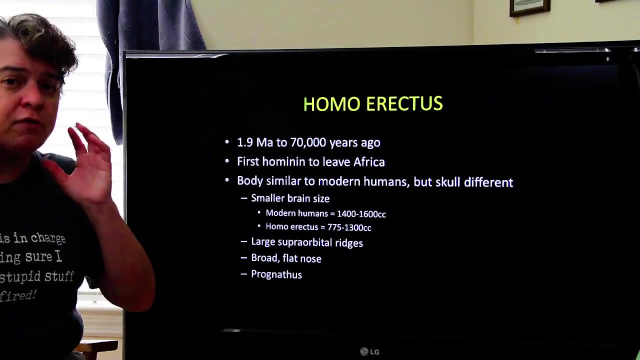 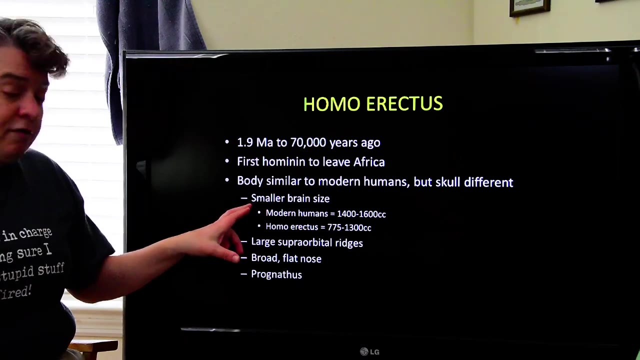 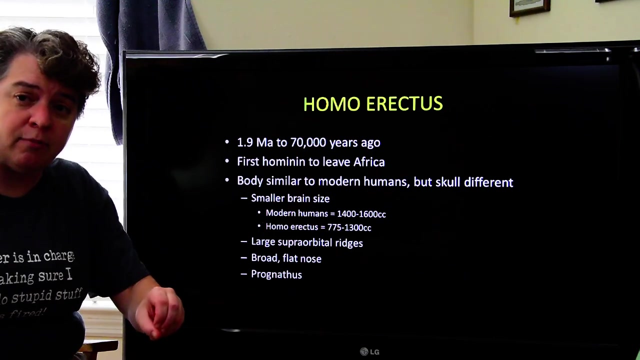 And this was the first of the hominins to leave Africa, And its body was very similar to modern humans, but its skull is different And the skull still retains some of the earlier characteristics. It has a smaller brain size, So modern humans' brain is typically 1,400 to 1,600 cubic centimeters. 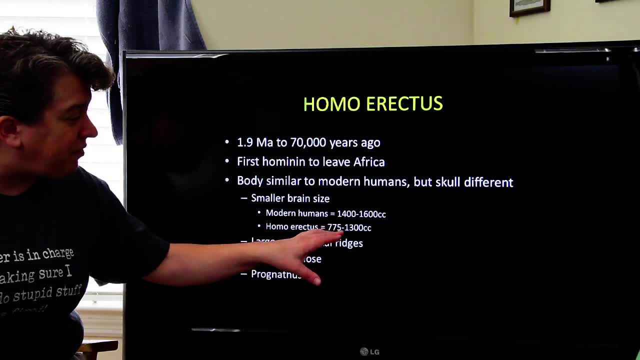 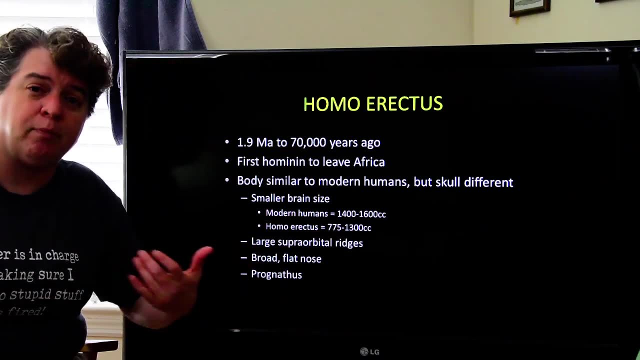 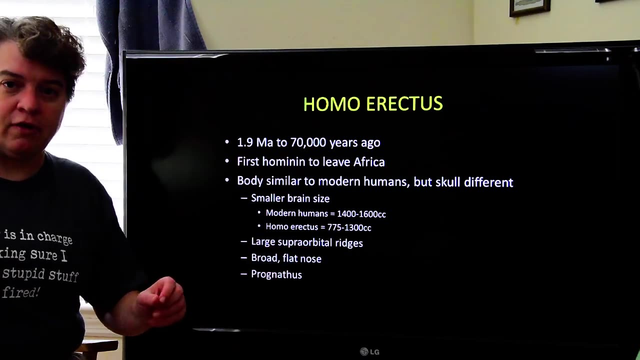 In Homo erectus it was about 775 to 730.. So it's about 1,400 cubic centimeters. So even at its largest it was still smaller than the typical modern human's brain. It has supraorbital ridges that are quite big. 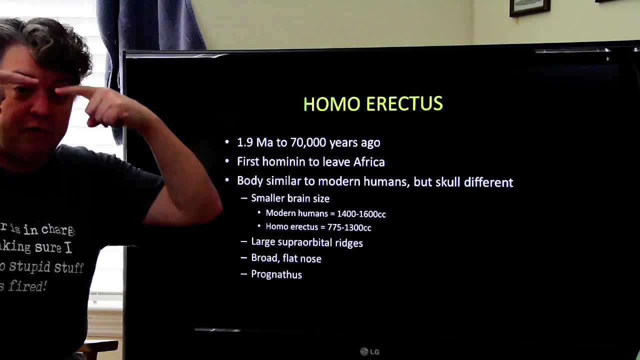 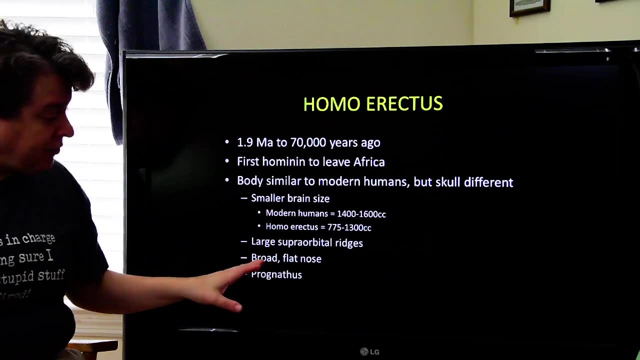 Now, when we talk about the orbits, that's where the eyes are. Supraorbital means above that. So there'd be these big ridges above the eye sockets. The nose was going to be broad and flattened And it is prognathous. 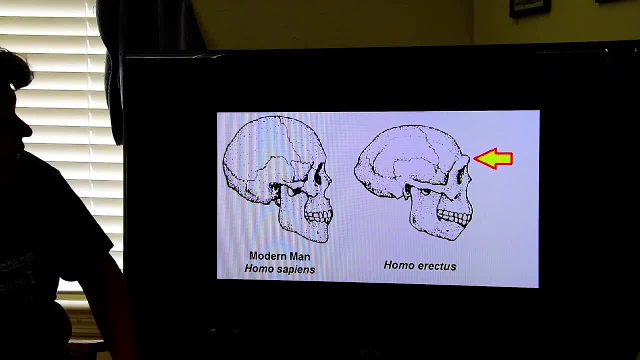 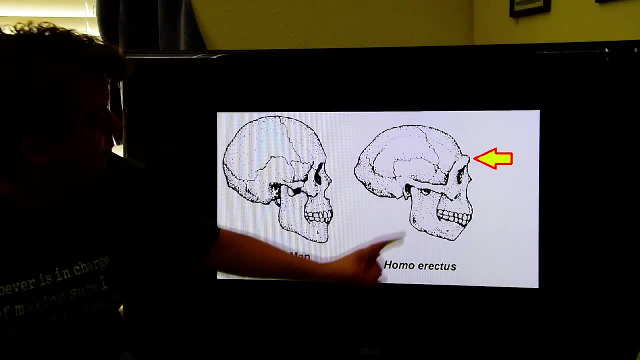 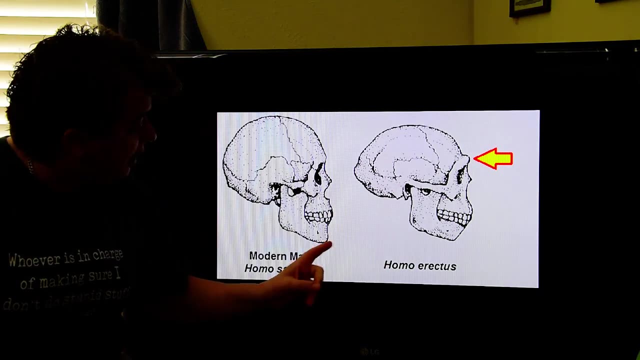 And I'll show you in a moment what prognathous means. Okay, So this is a modern human skull. This is Homo erectus. Now there's that brow ridge that I'm talking about, those supraorbital ridges, And then that prognathous. 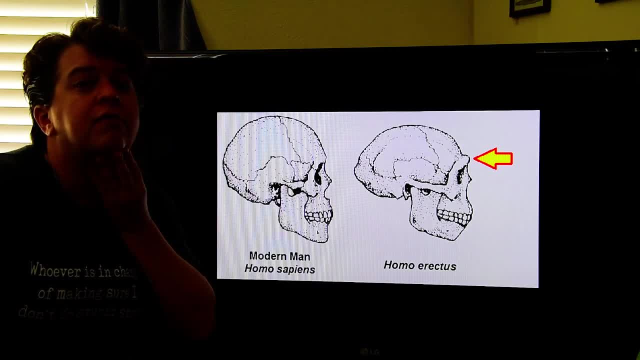 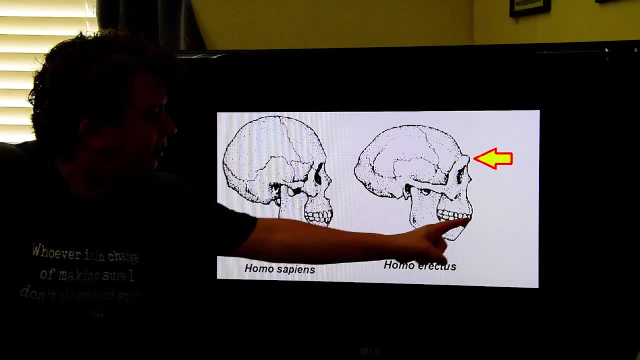 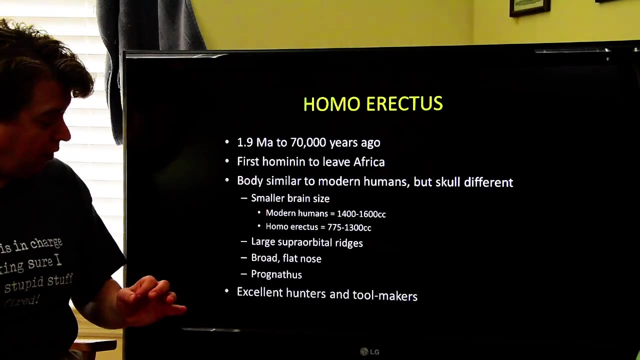 Do you see how the chin kind of goes backwards? That's what prognathous means. So in a modern human it kind of comes forward a little bit like that Prognathous In Homo erectus, And so that's some of the little differences that you would see in the skull. 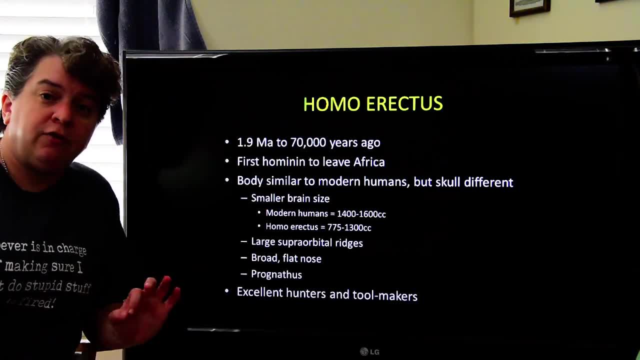 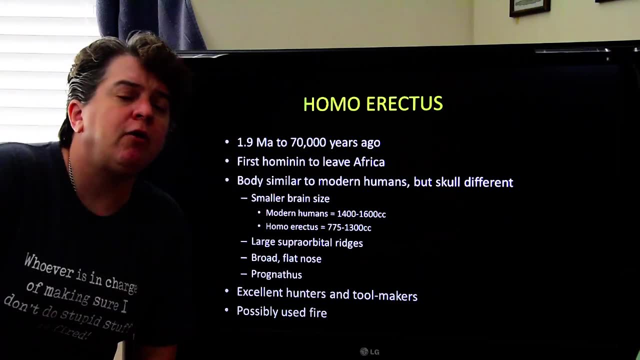 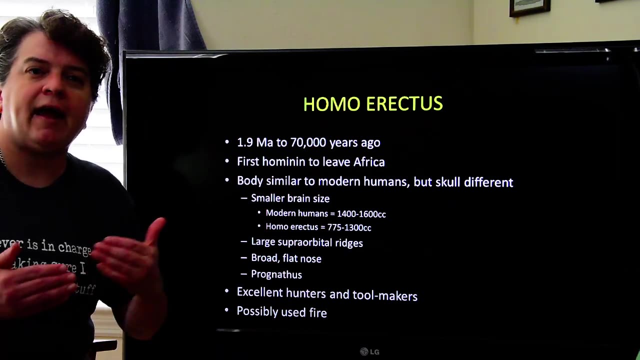 Now, these guys were excellent hunters and toolmakers And they might have used fire. I put possibly there because in some locations where we have Homo erectus there is evidence that there was fire, But we can't tell whether it was like accidental right. They came across a wildfire And had it. There's not that. you know, when people repeatedly use fire, you tend to get a hearth And you tend to get numerous fires on top of each other. We don't see that. 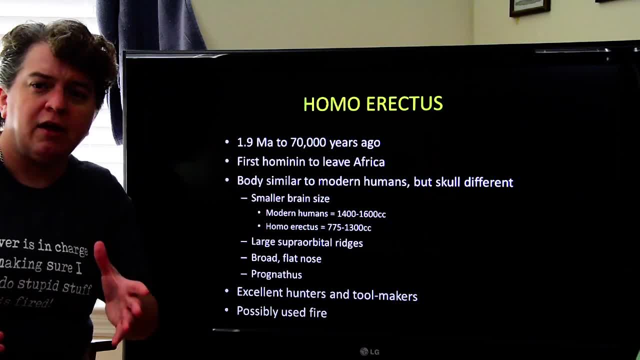 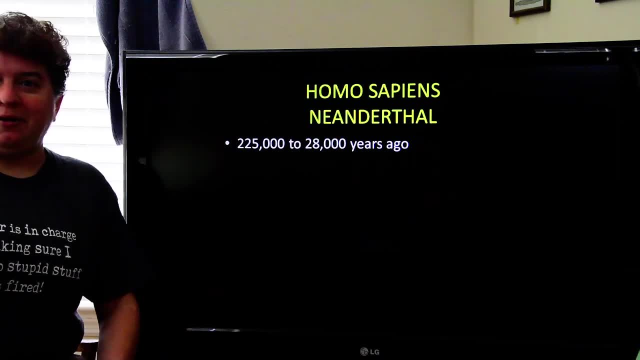 But we do see some evidence that sometimes fire was present with these guys, So they might have known how to use fire. Okay, We'll come up to Neanderthals in volume two. 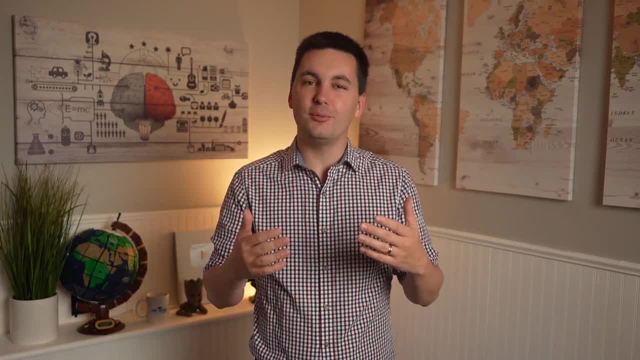 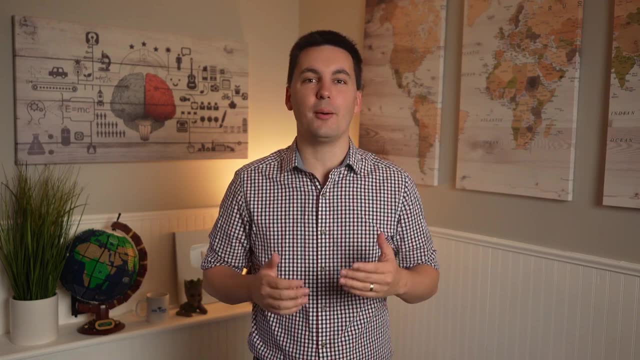 Hello there, geographers, and welcome back to the Mr Sin channel. Today we're going to be looking at the different political, economic and cultural effects of migration. As always, remember, if you find value in these topic review videos, don't forget to subscribe and check out some of my other resources in the description of this video. 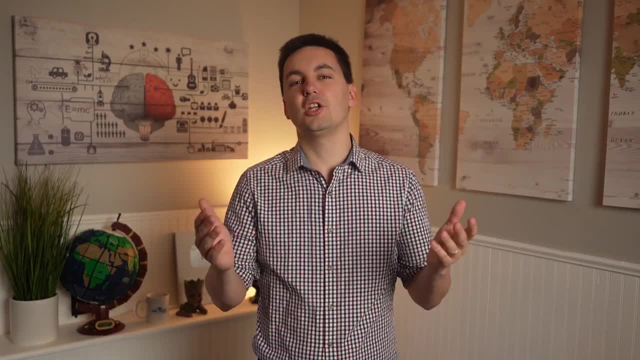 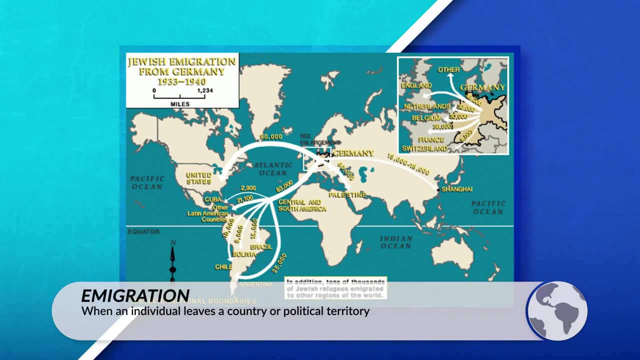 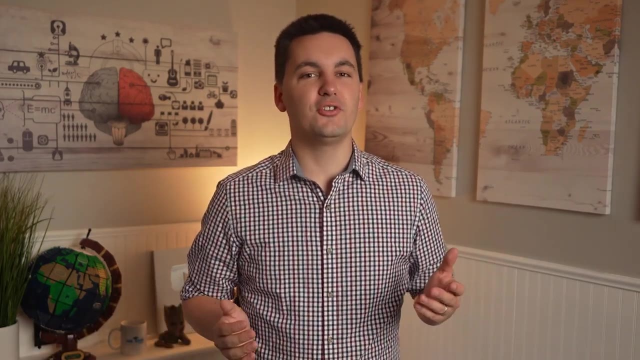 Migration has a variety of different effects on a society. We can look at historical events such as the Holocaust, which forced thousands of Jews to emigrate from Germany to different countries around the world. This forced migration not only reshaped the demographics in Germany and much of Europe forever, but also impacted places such as the Middle East.